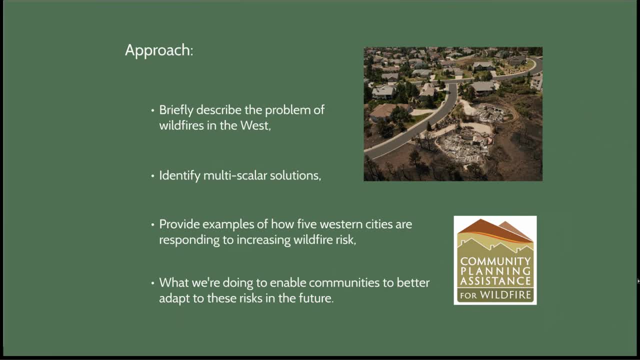 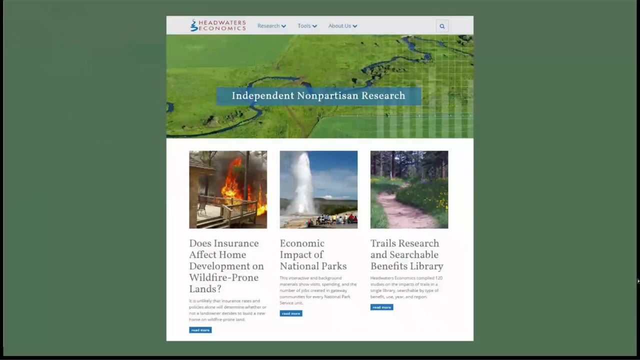 or Ready Set Go in that again, it focuses very much on a smaller niche of the larger arsenal of tools out there that are available, And I'll talk about that in a bit more detail as we move on. I work with a group called Headwaters Economics and we are a policy and research think tank based in Bozeman And over the past 10 years we've really specialized and honed in on some of these fairly wicked and complex 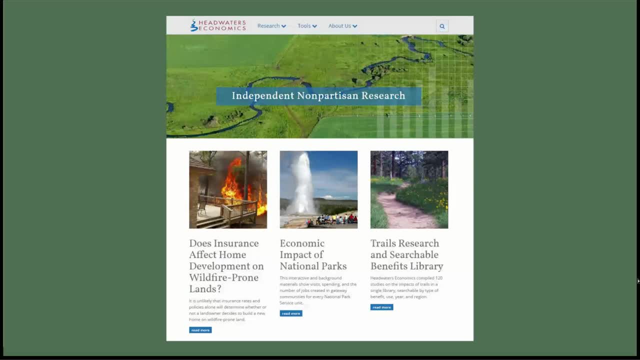 issues facing the American West, And by that I'm referencing the 11 states situated west of the 100th Meridian. So we've looked at everything from trails and recreational impacts to energy and coal development, landscapes to economic role of public lands and national parks And, in the area that I work in most specifically, is looking at the cost and impacts of wildfires, again in these 11 Western states. But rather than canvas this over kind of 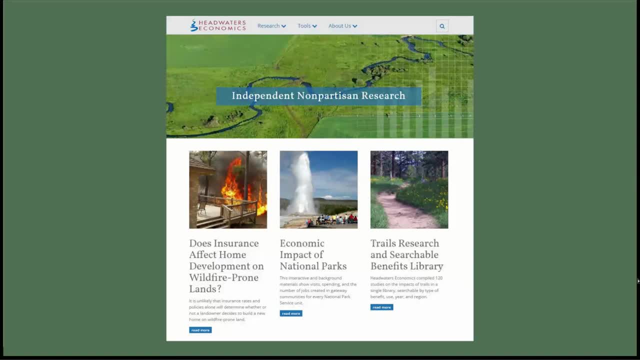 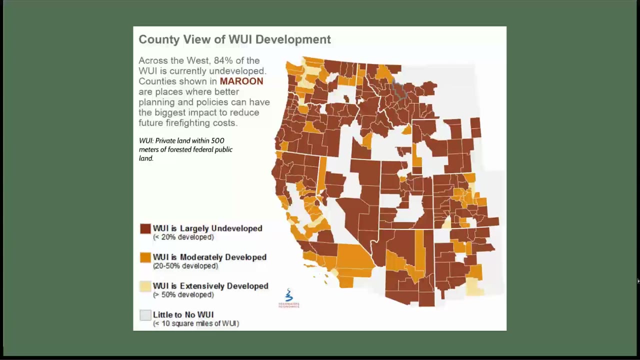 to to, even though you know the American West in general, we really want to focus in and specialize on certain geographies to make it a bit more detailed and and, quite honestly, a bit more tangible to grapple with this issue of wildfire, And so to do so, as Facey said in the introduction, we focus more specifically on the wildland-urban interface, or the WUI, And at Headwaters, based on analyses that we did in 2013,, and using the definition of the WUI as private lands situated within a 500-hectare. 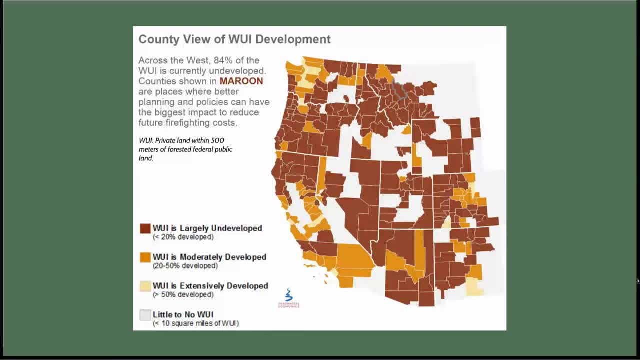 100-meter distance of forested federal public lands And, according to our analyses, what we came up with was that, in large part, the WUI is actually fairly undeveloped at this point within, again, these 11 western states. But rather than look at this as a positive note, saying like wow, this really isn't. 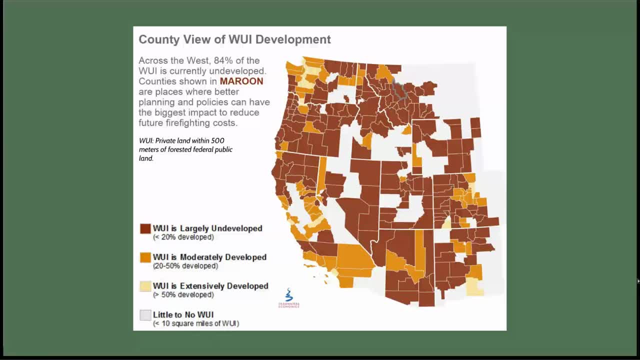 the issue that a lot of people say it is the WUI is really only 16 percent of it is WUI. We kind of turn it on its head and we say, well, that might be true, but really the potential for growth within the WUI is fairly significant. 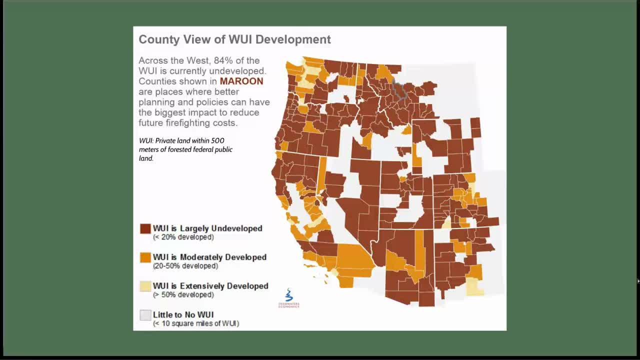 This is where growth is going to be directed in the short-term future, So in the 10 to 20 years from now, 84 percent of the west has a significant potential for ongoing growth. So this is the area that we focus on in particular when we're talking about wildfire costs and 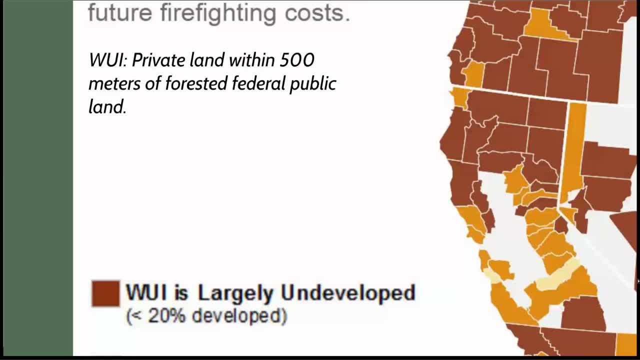 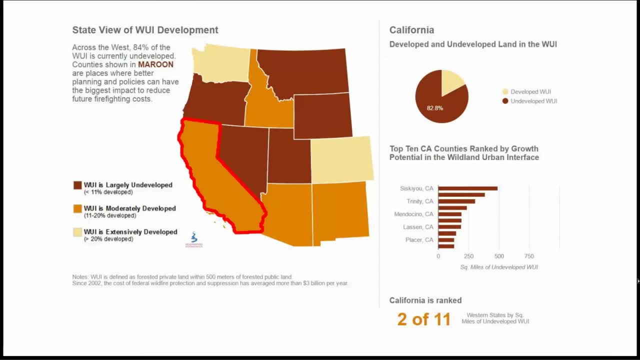 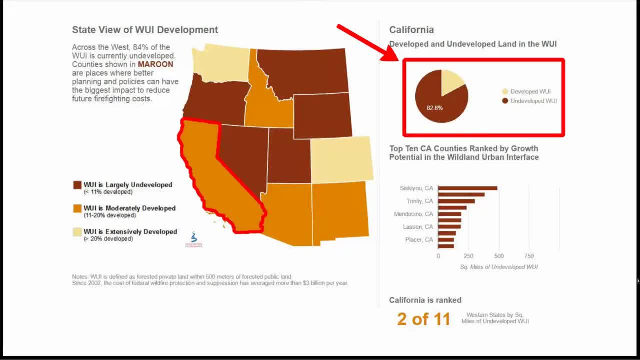 or 82.8 percent of it remains undeveloped, so less than 20 percent of it is developed at this time Again, and as I'll illustrate with the case of San Diego, this just suggests how much potential there is for growth within the targeted geographic scope. 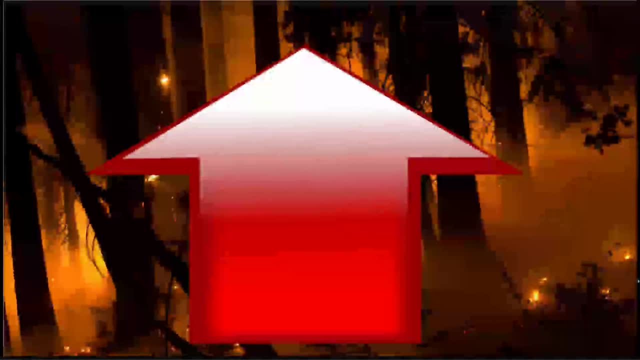 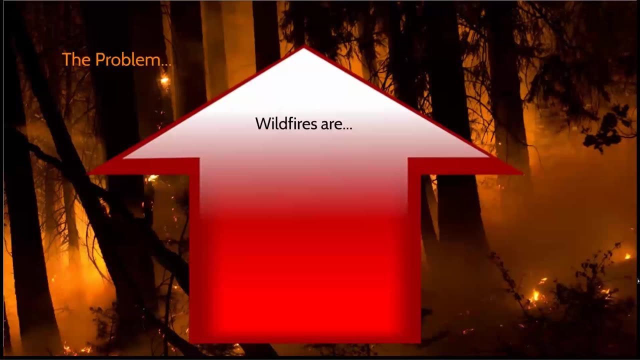 Very quickly running into why we have decided to look at land use planning with respect to wildfire risk. Again, this isn't the obvious answer. We're looking at the 10 to 20 year scale. We're looking at the impact and trends over the past 10 to 20 years. 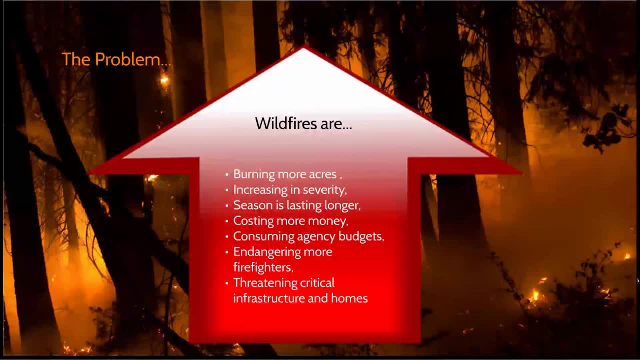 It's quite clear that this is an unsustainable issue, given current and predicted trajectories. Wildfires are burning more acres than they have in the past- 10.1, as in 2015.. They're increasing in scope to varying scale. in general, Seasons are lasting longer. 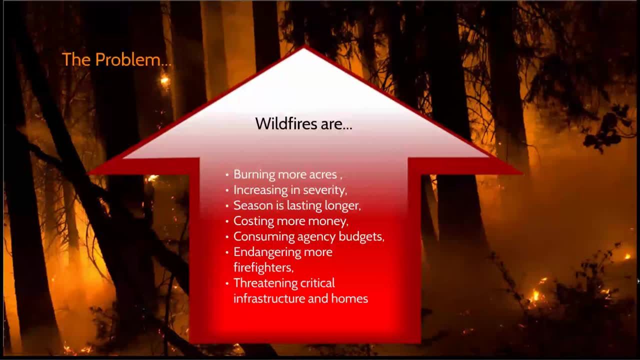 This is costing more money, which leads to fire borrowing, and programs such as the wilderness or recreational programs become sacrificed at the expense of fighting fires, increasingly engaging more firefighters lives and then threatening critical infrastructure, watershed homes, structures, etc. etc. Just looking at one. 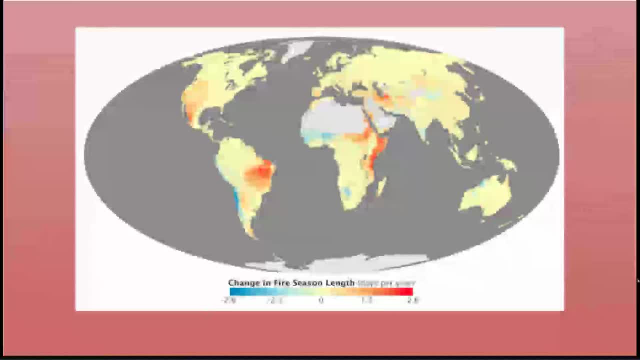 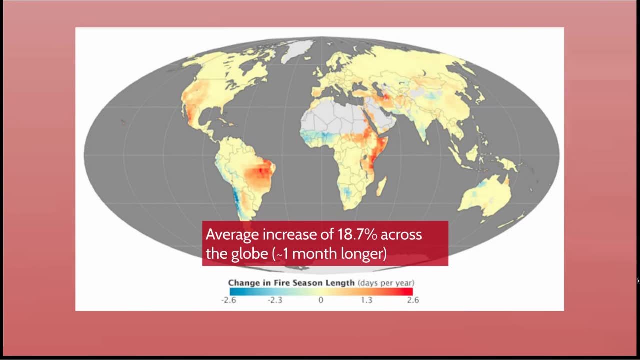 of these trends in a bit more detail. for example, and a study that came out of the University of Montana's fire science lab- was that, on average, wildfire seasons are lasting eighteen point seven percent longer, or about one month, and so what this implies is that fire seasons in general are coming a little bit earlier. 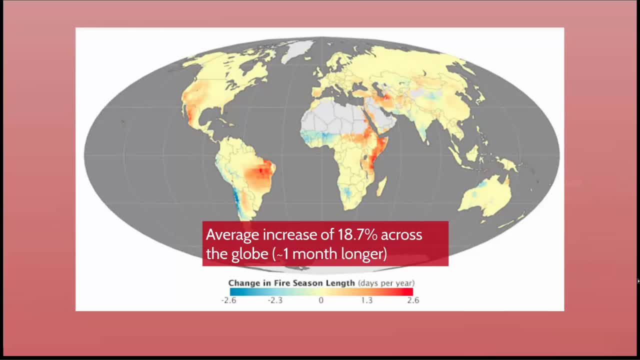 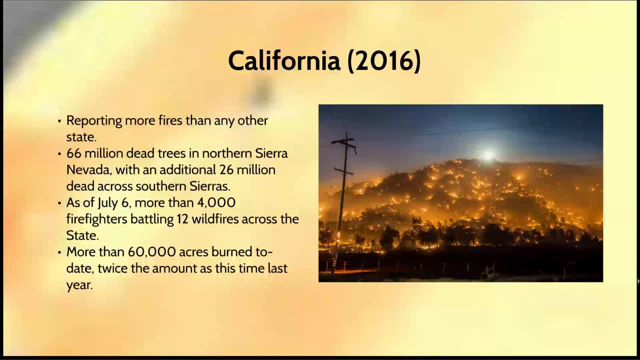 in the spring and they're lasting a little bit later into the fall. Looking again, just as California, as an example of how this might manifest, and looking most recently within the 2016 year- fire season year, rather- is that fires- California as a state is reporting more fires than any other state right now, and 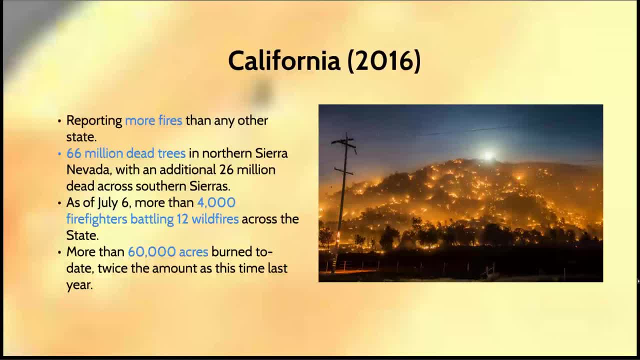 that this is potential for growth, given a recent study indicating that there's vast areas requiring fuel treatment: Sixty-six million dead trees in the northern Sierras and 26 million estimated in the southern Sierras- Again, a lot of potential for fuel buildup within these landscapes. As of July 6, which I believe, 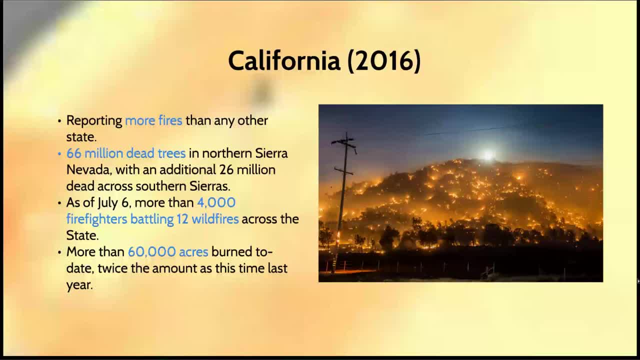 is kind of the peak of what it's been so far this year. there was 4,000 firefighters battling 12 large wildfires and so far, more than 60,000 acres have burned, which is more than twice the amount this time last year. As we all know, 2015 was fairly significant in itself, so you 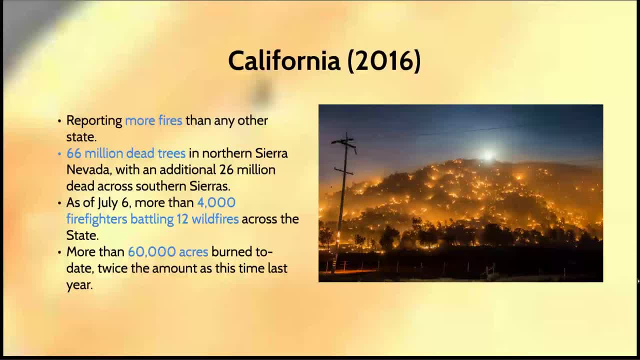 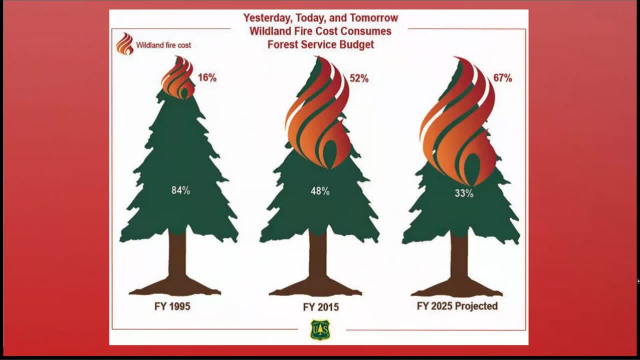 know again, given these trajectories, it is an issue on how this directly impacts, you know, in terms of economic costs, is by looking at the Forest Service budget. This graph infographic is a cost comparison of over just a 10-year time span and, as you can see, in 1995, 16% of the overall Forest Service budget was going towards wildfire. 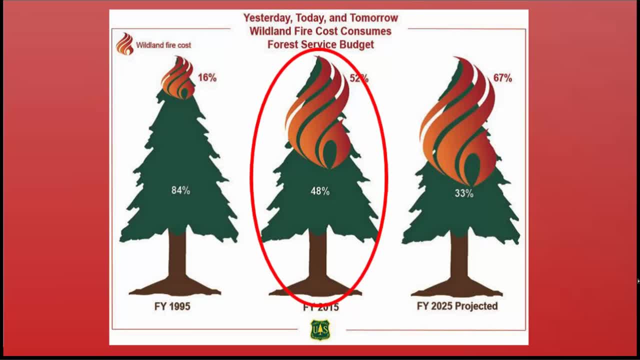 As of 2015, this had increased to 52%, and this whole this 52% means both fire prevention and preparedness programs, as well as post recovery. In 2016, this has already increased by 4%, so now we're looking at 56% of the overall Forest. 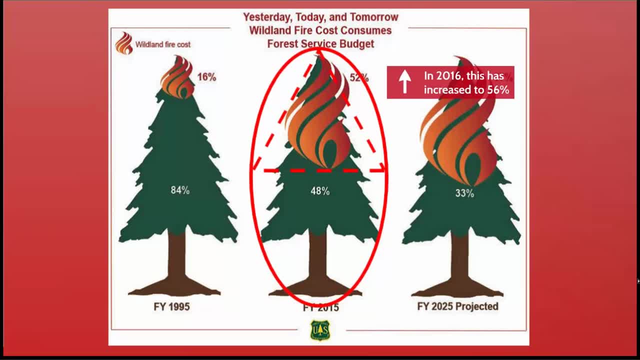 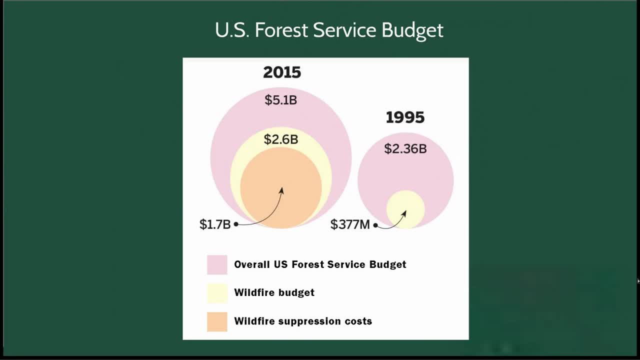 Service budget is going directly towards wildfire. Breaking it down into a bit more itemized detail again was across comparison over 10 years. you can see that in 2015, 16% of the overall Forest Service budget was going directly towards wildfire. 2015, the whole Forest Service budget came to $5.1 billion. 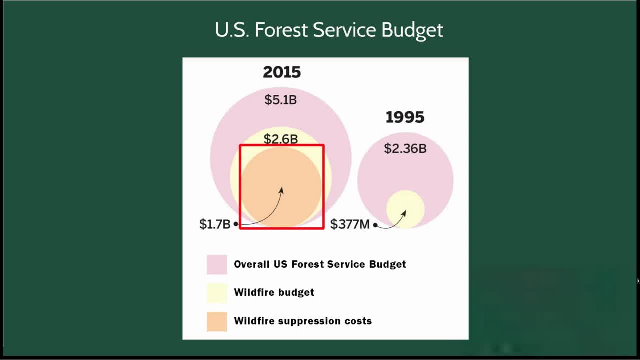 Of that, $2.6 billion went directly towards wildfire. but breaking that down even further, $1.7 billion went directly towards wildfire suppression or the costs that are required to actually put fires out for the protection of lives and homes. Again, it's unsustainable if you start to look at the long-term trajectories. 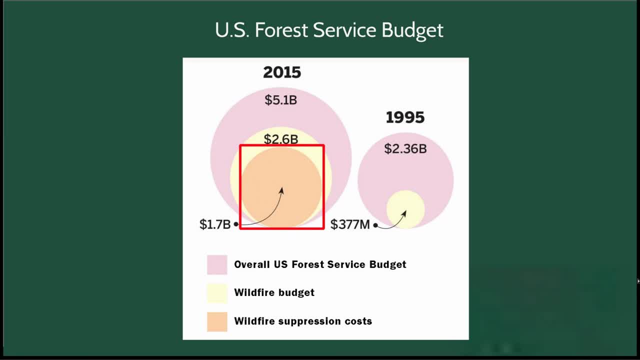 They're saying by 2025 that the Forest Service could be consumed 67% by just wildfire costs alone. This again comes at the sacrifice of other programs within the Forest Service. If you're looking at the 2016 budget, it's grown to be $5.6 billion and of that, 56%. 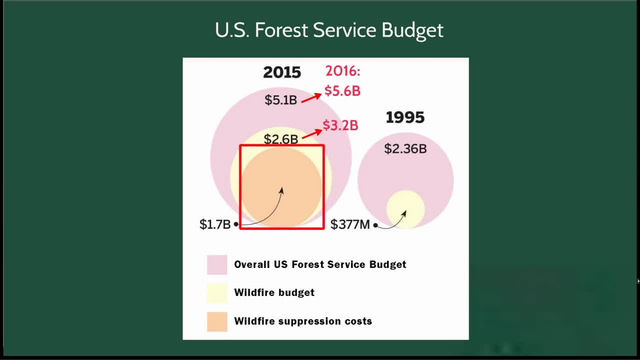 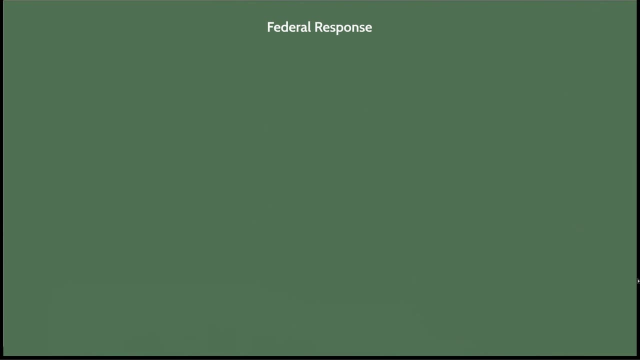 or $3.2 billion, is going directly towards wildfire. This is an issue, certainly for the federal agencies, And how money is going to be appropriated and allocated into the future. Looking at how the government has responded in the past, in 2009, they passed a bill called 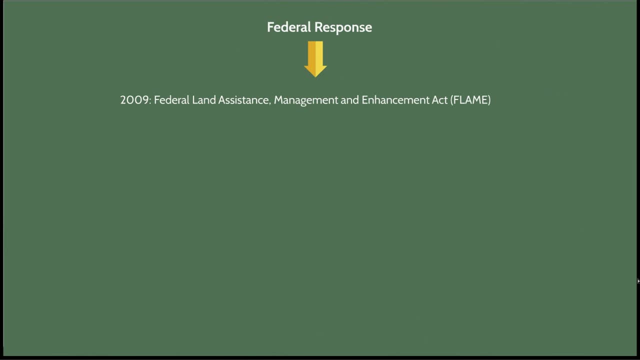 the Federal Land Assistance, Management and Enhancement Act, known as FLAIM. What this piece of policy did was really try to target how wildfires are going to be addressed, both on the ground as well as the overall administrative and bureaucratic level. What came out of it was the most immediate deliverable. 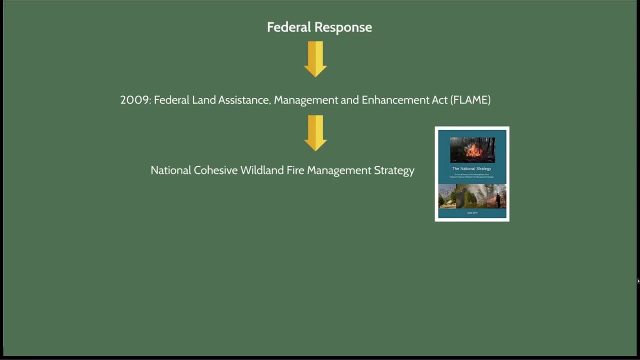 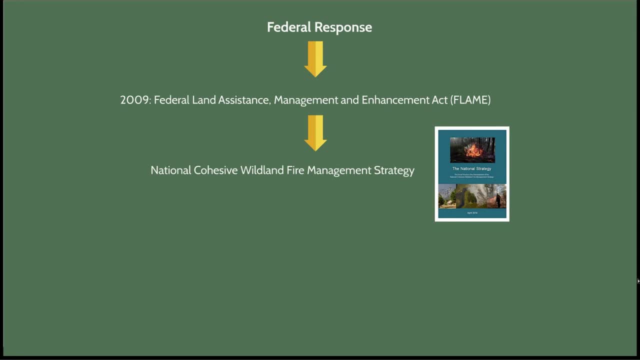 What came out of that deliverable was a document known as the National Cohesive Wildland Fire Management Strategy, Or the cohesive strategy, as it's often shortened to. This document outlined three very specific pillars that were going to be addressed. The first one looked at restoring and maintaining resilient landscapes in wildfire prone areas. 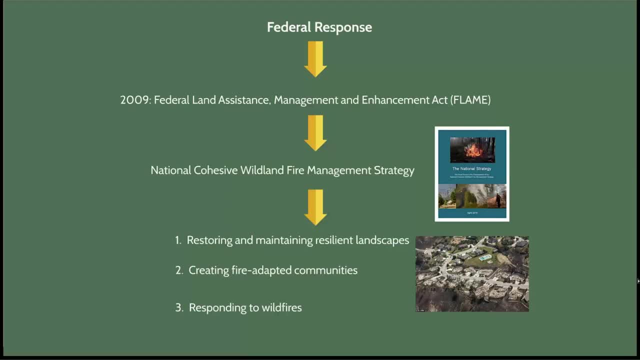 The second one wanted to address the creation of fire adapted communities in wildfire areas, And the third one really focused on the community, And the fourth one focused on the tactical, operational responses of wildfires on the ground, And so what we at Headwaters wanted to do was to look at this idea of creating a fire adapted community. 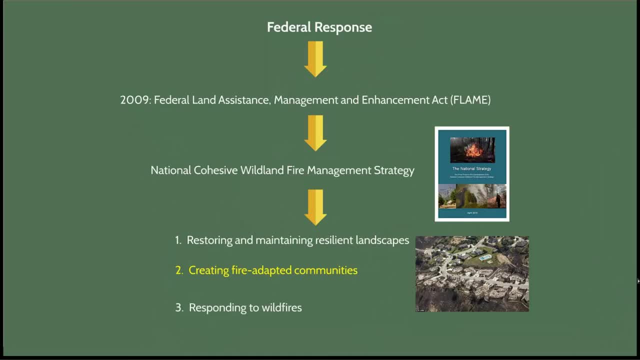 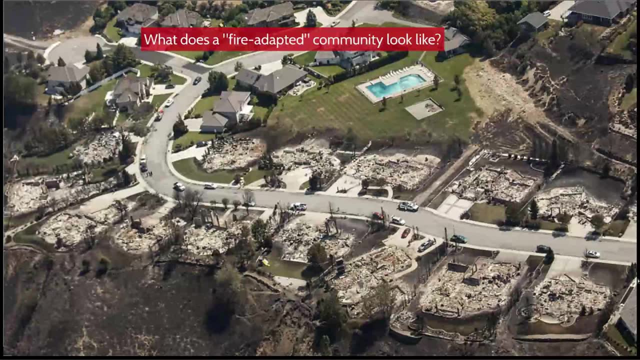 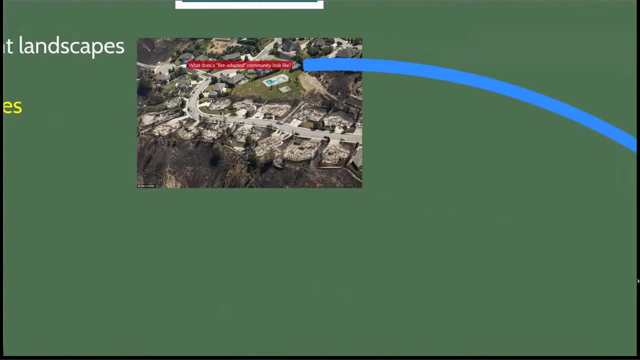 And we, along with others, were really curious: well, what does that mean? What does a fire adapted community look like when it actually manifests in communities in real terms? And so what the government did was they kind of broke it down into these kind of principles. 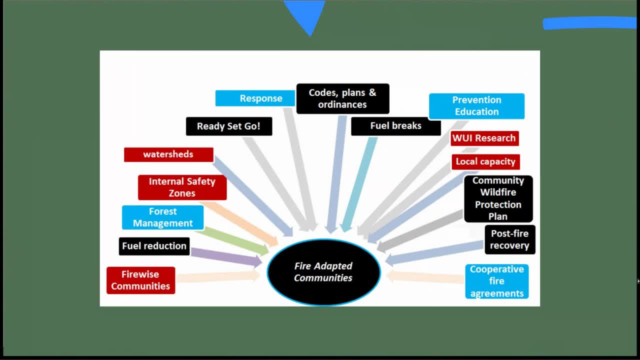 And fundamental elements of what sustained a fire adapted community. And so, again, they developed these programs such as FireWise, Ready, Set, Go, the FLAC or the Fire Adapted Communities Learning Network, And all of them were really focused on not only the communities but the home ownership. 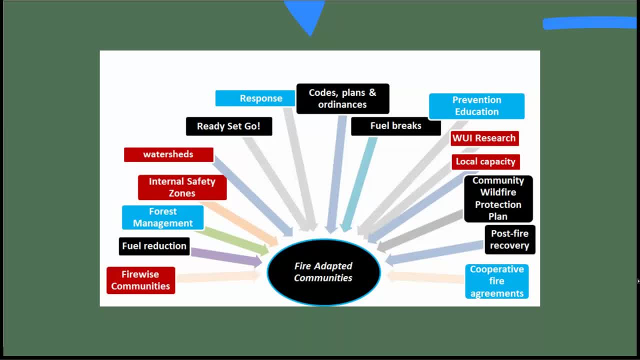 role and trying to raise overall public awareness. Also, part of this is that they honed in on plans such as community wildfire protection plans, Looking at post-recovery efforts, WUI research, And so it's really broad and diverse. But the one thing that stood out to us on a bit more practical terms was this top consideration up here of codes, plans and ordinances. 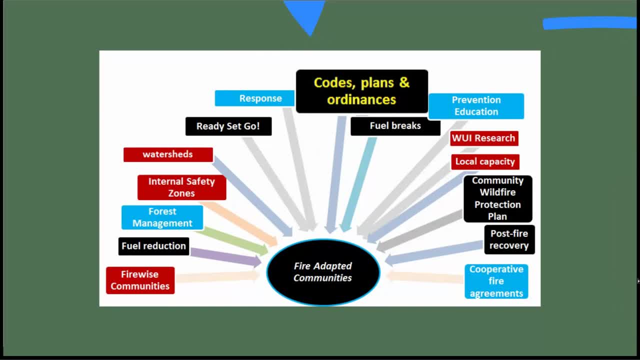 And Headwaters Economics really wanted to know a bit more about that And what does that really mean, Because nobody really started to dig into this really deeply and figure out how that could be applied in a really practical, realistic manner. So that's what we did. 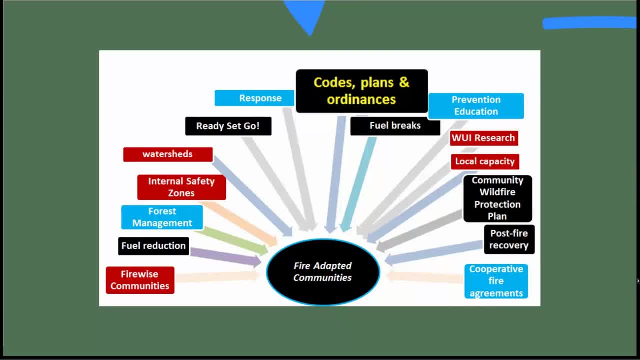 And so the program and our efforts that we've done with respect to looking at codes, plans and ordinances are really intended to be complementary to these ongoing and existing programs such as FireWise or the FLAC Learning Network. There's not supposed to be overlap there. 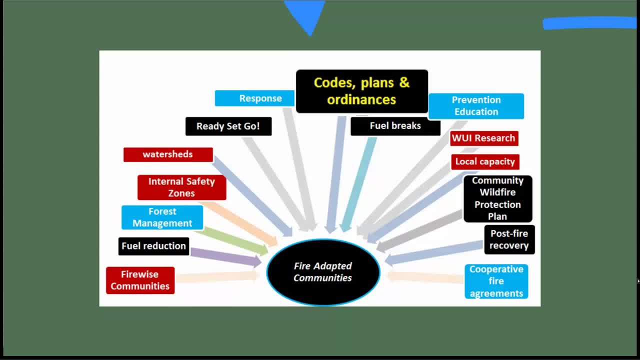 And we're really trying to work together in a parallel partnership which, so far, I would like to think, has worked well. So, again, this is the area that we have specialized in and really willowed our efforts into, So it's more particularly at how this can be implemented at the community level. 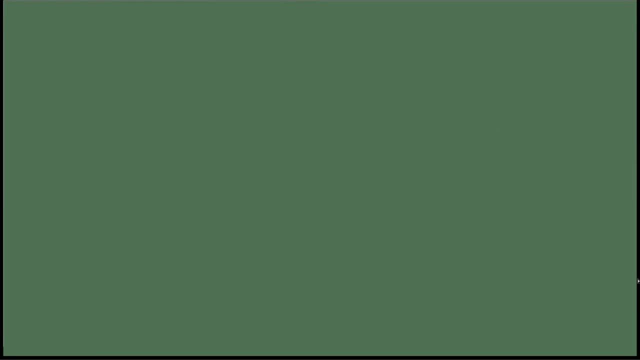 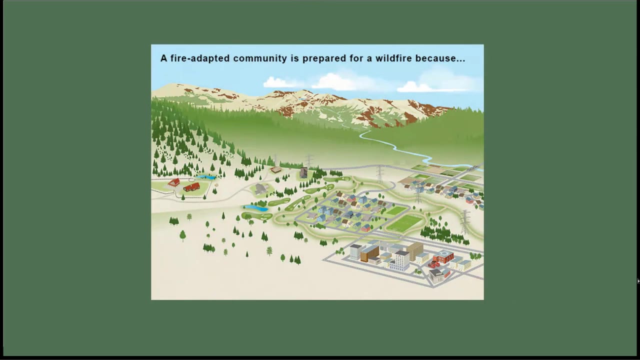 And in order to do so, I should jump ahead here really quick, Wanting to look at what we mean by when we're thinking about. what does land use planning look like in a fire adapted community to reduce wildfire risk? And so we call this graphic firetopia, because this is generally an ideal world where you can work with a community that's situated within the WUI. 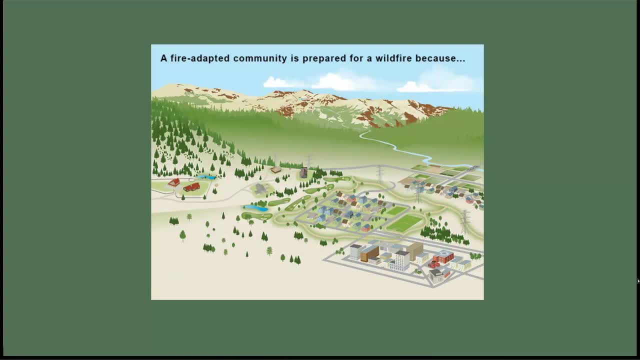 and have some sort of control over how that community is designed with respect to land use planning strategies, It would become more fire adapted than if it didn't incorporate some of those land use planning tools. So, for example, this is a community- again very hypothetical, but often it's demonstrative of what many communities in these western states look like. 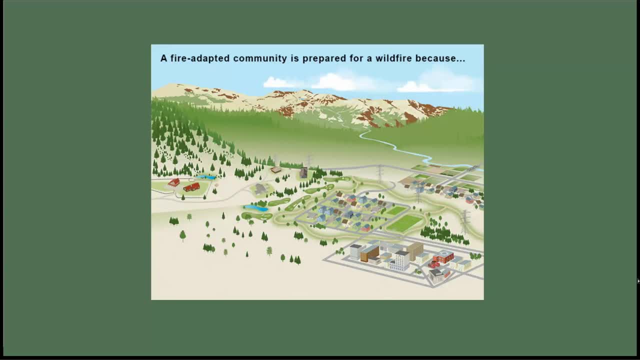 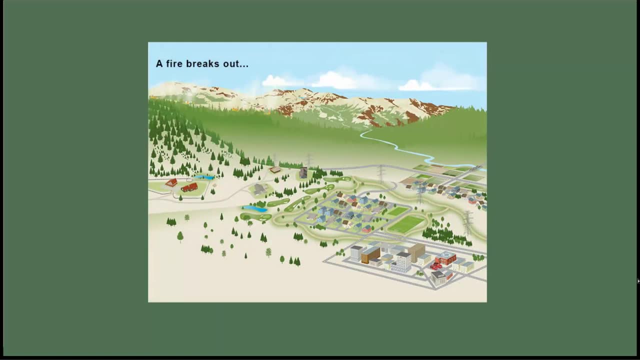 It's not far from a forested area, There's a watershed in the distance And it's primed for ongoing growth. And so, given this kind of scenario, and a fire breaks out up in the forested landscape and, given prevailing winds, quickly starts to approach the community. 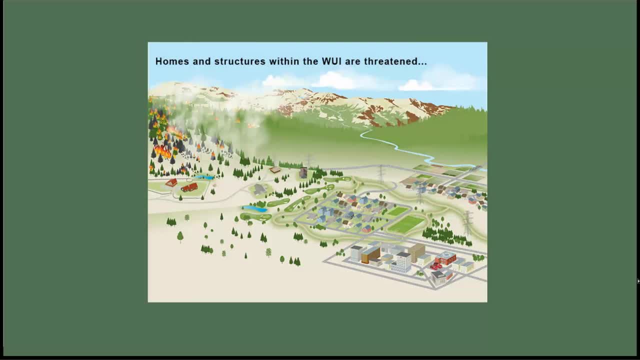 threatening those homes most immediately situated within the WUI, but then also threatening those homes that are situated just outside, through ember spread and flame enhancement. So as the fire starts to move down, slows increasingly getting closer to the communities. there are certain things in place that the community has planned. 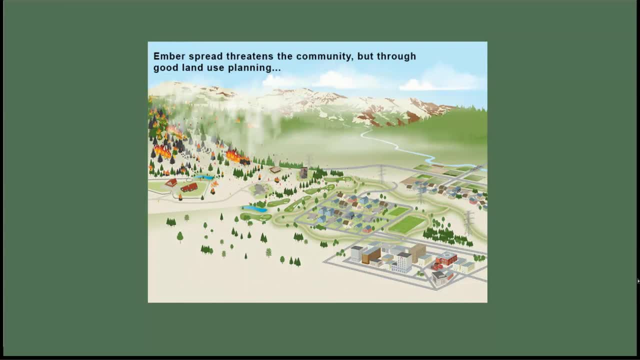 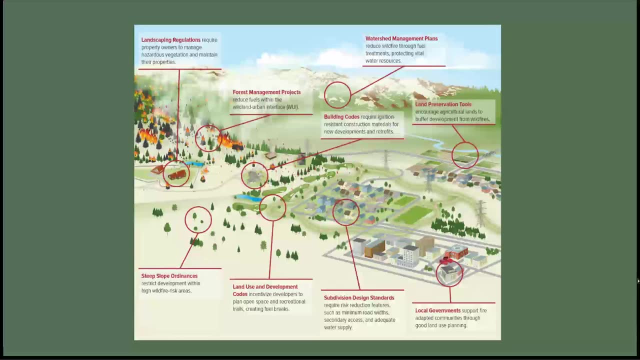 around a possible wildfire disaster or catastrophe And, in doing so, these communities and these homes are already set up to anticipate a wildfire event. For example, you have fuel treatment areas close to the WUI. You have homes that are situated proximate to those high-risk areas requiring certain hardening materials. 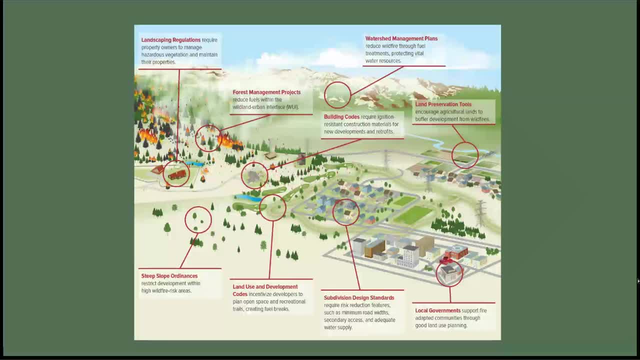 Metal roofs or the decking or the venting materials have to be a bit more fire resistant than what we're used to And what's traditionally used in those areas. You have golf courses and irrigated lands or bike trails serving as fuel breaks and buffers from some of those immediate fire threats. 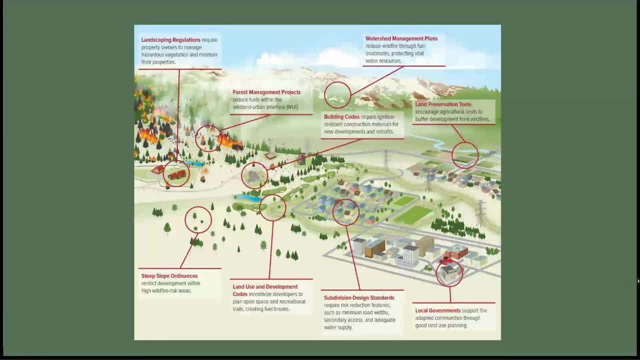 And even the design of some of the subdivisions have been manipulated to integrate wildfire risk. For example, they have multiple ingress and egress routes, So accessibility It's condensed housing, There's vegetative landscape treatment, And so this differs from how much of what we're used to. 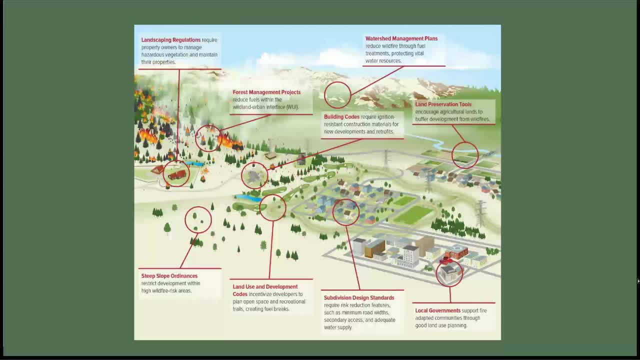 It differs from how modern subdivisions are often designed within the WUI, who have a one-way in, one-way out. They're commonly referred to as suicide subdivisions for that reason, And so it's actually looking at design principles of how a development can take place in some of these communities to better integrate wildfires. 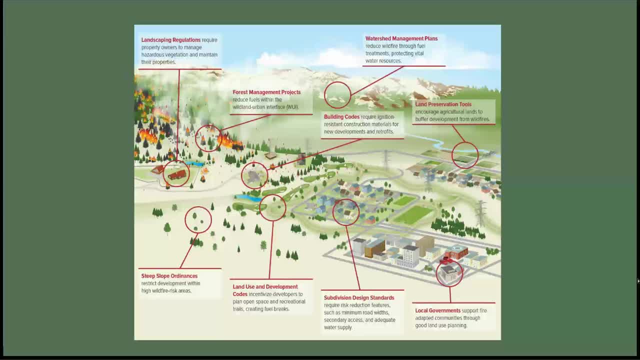 So this is again what we hypothetically refer to as firetopia and what we're working towards achieving. In order to see what that really meant, we worked with Community First in Summit County, Colorado, in 2013 through 2014.. 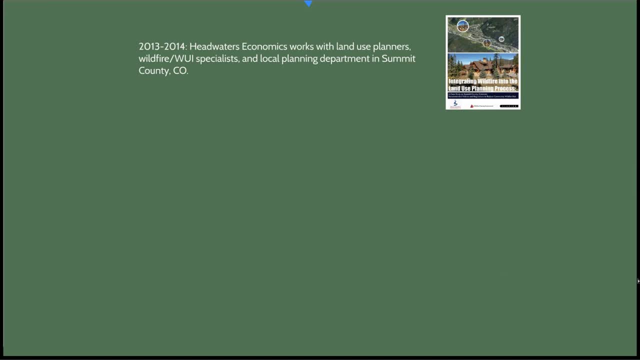 And this was a pilot study And we received funding from a private foundation to actually explore what land use planning meant with respect to wildfire risk, And so we worked very closely with the land use planners, the WUI specialists and the local fire departments in Summit County to go very thoroughly through their actual planning process and their development review. 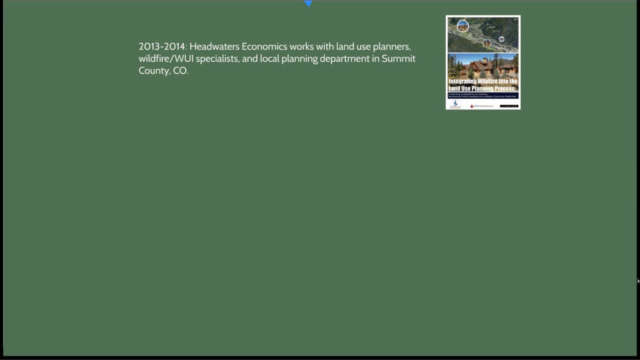 Strategy to see how could wildfire risk be better integrated into those frameworks. So it was everything from the placement of homes and view sheds to how landscapes were treated and some of the vegetative components in some of these subdivisions, And what came out of it was a set of recommendations that we provided to the county board of commissioners and of which, you know, 80 to 90 percent were integrated into both their short and long term planning outlook. 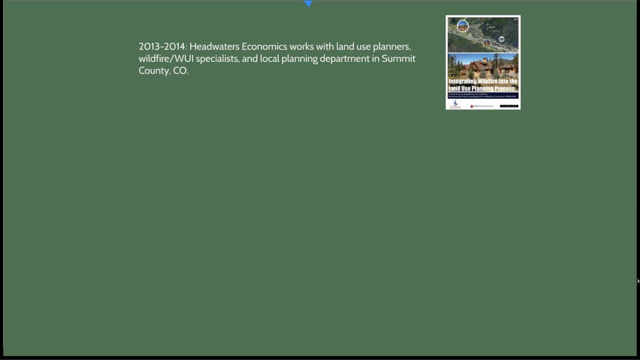 So we viewed this as a success And so we went back to the Forest Service and we requested additional funding to continue these efforts into five more communities throughout the West, So effectively scaling it up. So, through a cooperative agreement with both the Forest Service as well as our private funder, we were able to work in the communities of Austin, Bend, Missoula, Taos and Wenatchee. 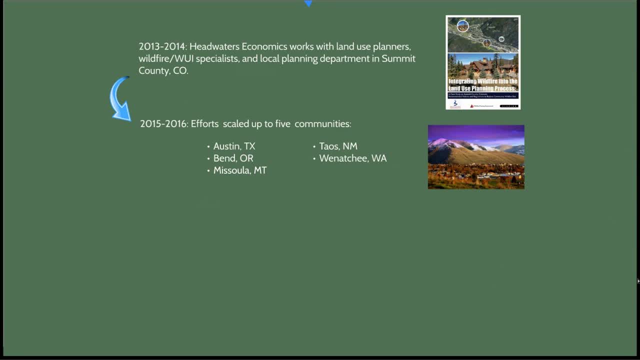 And so those are efforts that this is kind of the first phase that are ongoing and are anticipated to kind of wrap up Here by the end of the summer. But in addition to this, and in order to provide better context and understanding about what land use planning tools are available, was that we profiled five Western cities that were already applying fairly aggressive land use strategies to respond to this issue of wildfire risk and land use planning in the West. 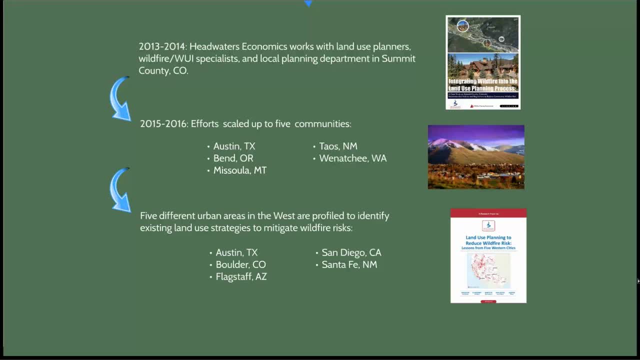 And so we looked at Austin, Texas, Boulder, Colorado, Flagstaff, Arizona, San Diego, California, And then Santa Fe, New Mexico, And that's what I'll really be talking about in a bit more detail here in the next part of my presentation. 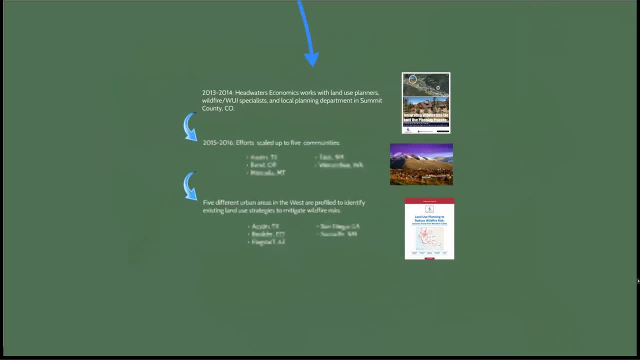 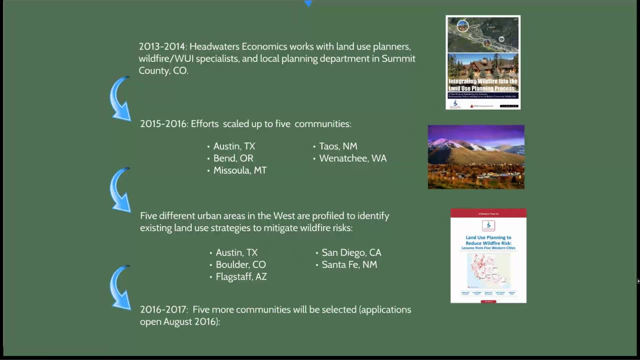 But then also, given this and ongoing efforts, we have received funding for work here in the next year- 2016 through 2017, to select five new communities to work with throughout the country, not just the West. So we'll be accepting applications for that program starting in August. 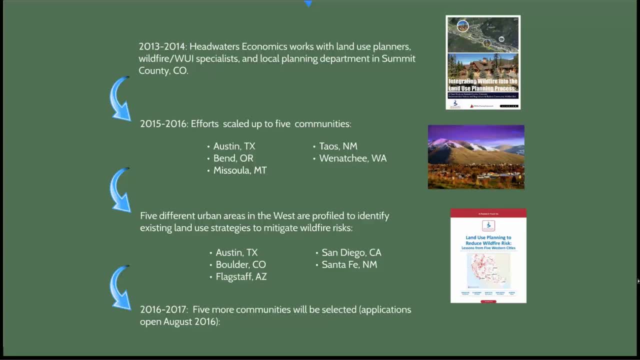 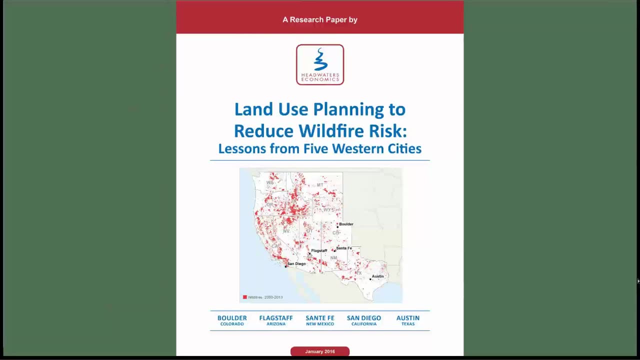 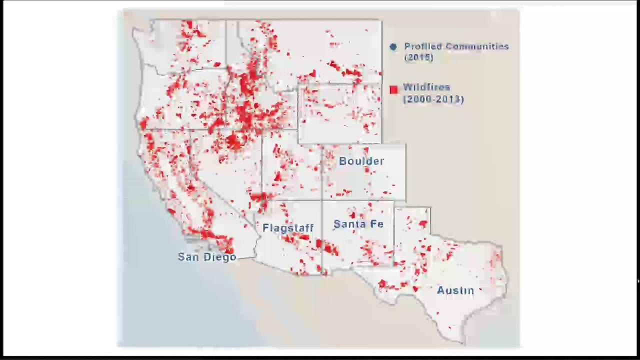 And I'll talk a little bit more about what the program actually entails towards the end here. But what I want to do now is just shift gears and highlight some of these land use planning strategies that came out of this report. Again, working with these five fairly progressive cities and what they're already doing to respond to wildfire risk. 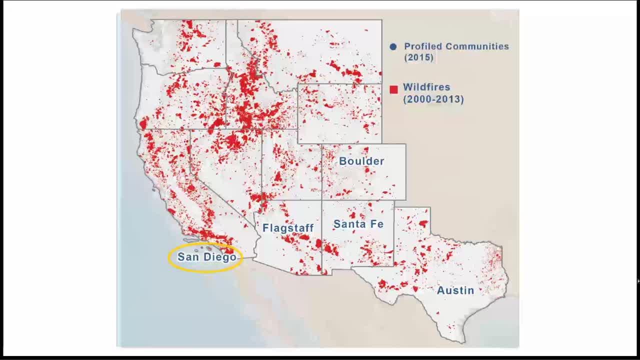 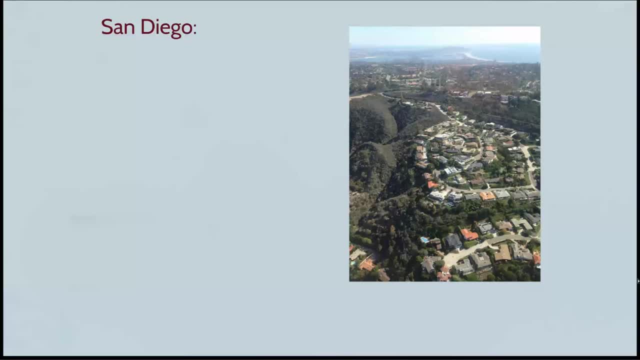 The first of these was San Diego, California, And San Diego is really interesting. just given the vastness of their WUI, It's incredible And from the air it's that much more illustrative. But they're new And the entire WUI measures about 500 linear miles across. 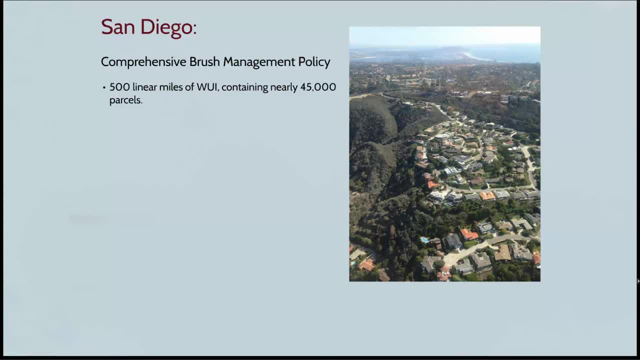 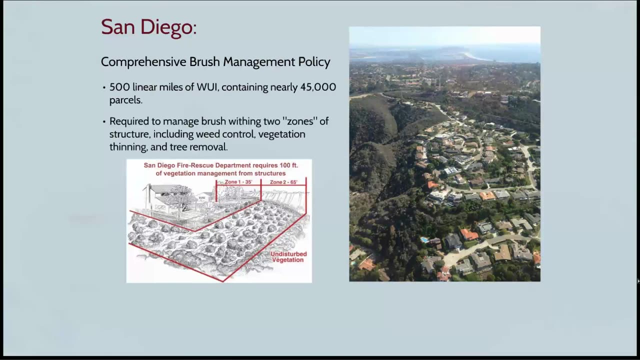 It contains more than nearly 45,000 individual parcels. So what they've done is implement a comprehensive brush management policy for all structures- habitable structures situated within that WUI boundary, And they actually have an on-site inspector go to each of these homes and ensure that the home has complied with this brush management policy. 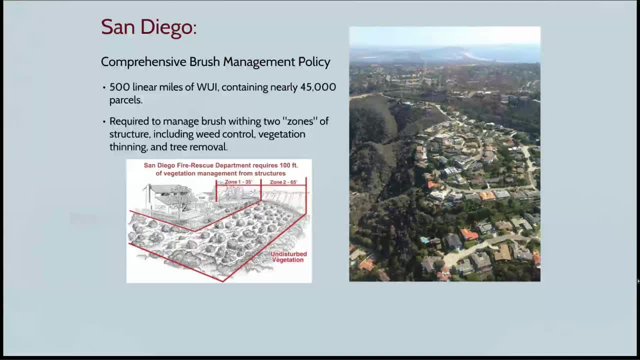 And what this breaks down is that for every structure they have to have a 100-foot vegetatively treated landscape area divided into two separate zones for a total of 100 feet. So the first zone is fairly intensive. It's going from the end of the habitable structure out 35 feet. 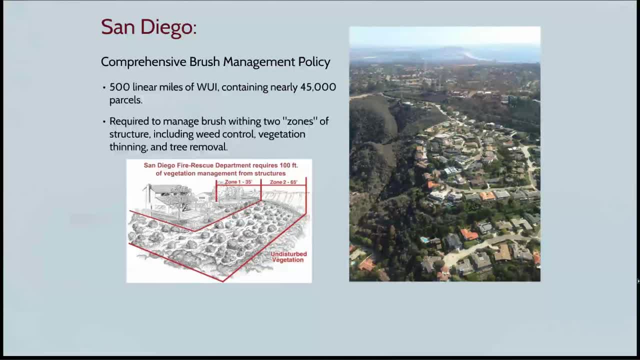 And so this requires certain tree removals if necessary, brush management of all shrubs, loose debris, weed thinning if needed, and overall kind of management and control, kind of management of that that area at a fairly intense level, and then the latter zone is 65 feet, so covering again that full hundred feet landscape area. 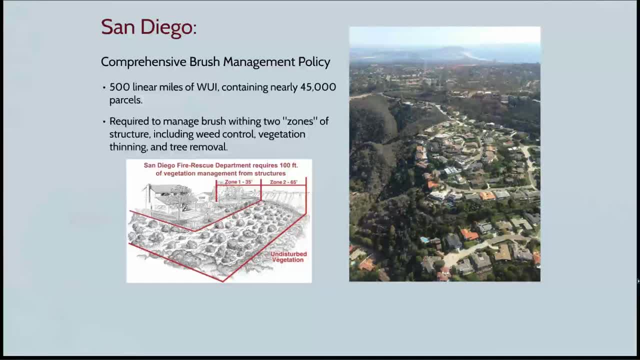 this is not quite as stringent here, but again does require quite a bit of management in terms of if there's certain trees that seem like they're dead are going to act as fuel load, they're required to be removed. shrubs and shafts, chaperone is needed. and then what's unique about this in San Diego is 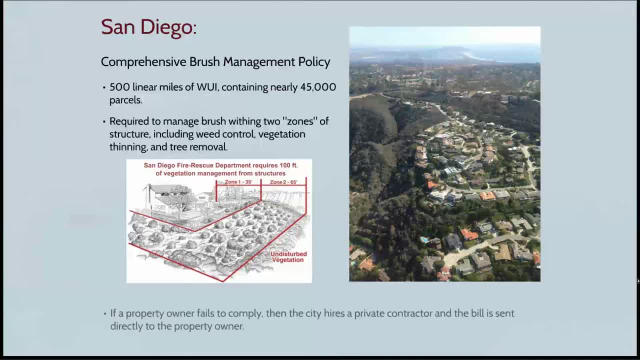 due to the on-site inspections of some of these structures. if the homeowner fails to comply with this brush management policy based on the on-site inspection, then the city actually hires a private contractor to go to that property and do it themselves, and then the city bills the homeowner the cost. 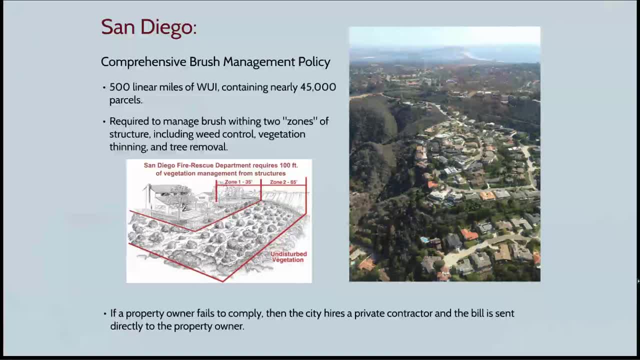 required to hire that contractor and if the homeowner still fails to comply, then a lien is actually placed on that property until payment has been received. so this is a way that San Diego has achieved really issues with respect to wildfire risk, not only for proposed new developments but existing structures. again a fairly progressive and 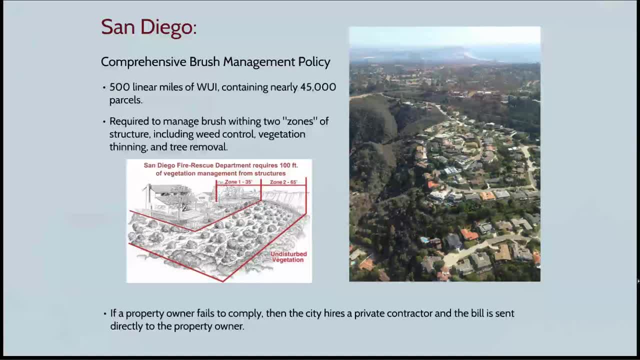 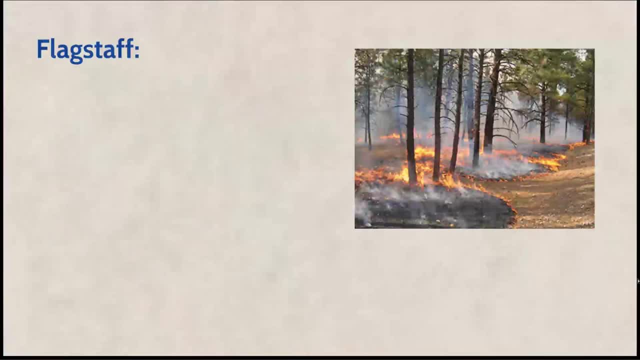 aggressive tactic to dealing with wildfire risk in that city. I'm looking now at how it flagstaff has done. flagstaff has built pretty much a city within a ponderosa pine forest- actually the most, according to some studies, the largest, most extensive ponderosa pine forest in the world. and so, given that they of course have very immediate wildfire, 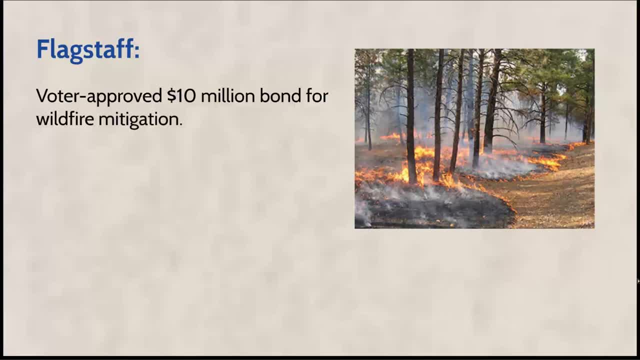 threat, and so what happened was: in 2012, there was a significant wildfire but, more importantly, a post wildfire flooding event in which a young girl was killed, and there was a significant economic loss due to that, not to mention direct impact to the watershed. and so the voters, the voters and actual citizens of 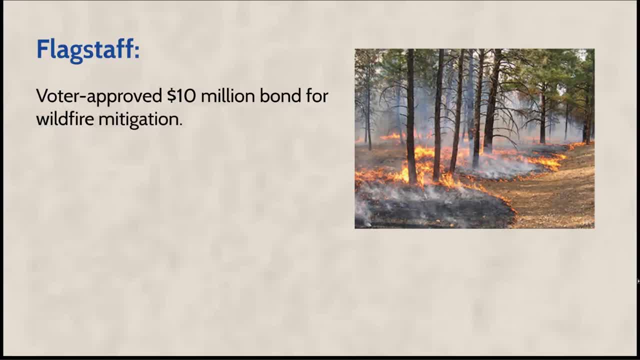 Flagstaff approved a bond and act themselves in order to have funds for a wildfire mitigation activities, and what this resulted in was actual fuel treatments taking place within the city limits, so unique in that the actual citizens recognize their own risk and awareness to that threat and agreed to pay for these treatment programs out of 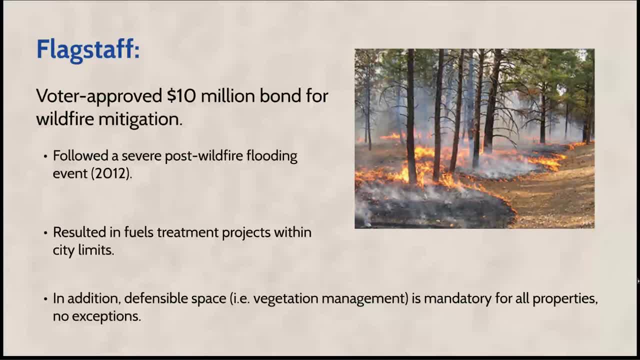 pocket effectively. in addition, because of the the presence of the ponderosa pine forest, homeowners are required to have essential space. no exceptions if you live within city limits, and so there is no. unlike San Diego, where it's a hundred foot zone, in Flagstaff it is from the end. 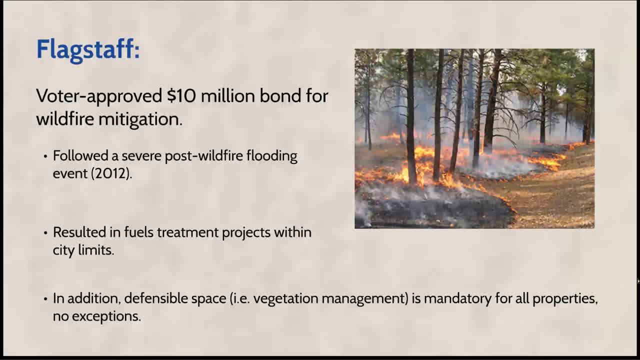 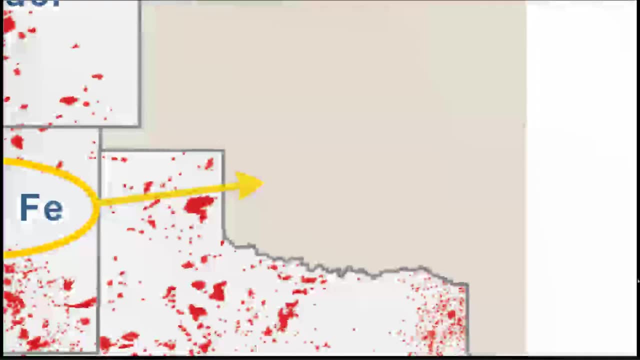 of your structure to the end of your property line, irregardless of how big or how small that might be. so that too is a fairly unique and progressive way of approaching wildfire risk within Flagstaff, quickly profiling the next city. we have Santa Fe here, Santa Fe as a southwest fairly. 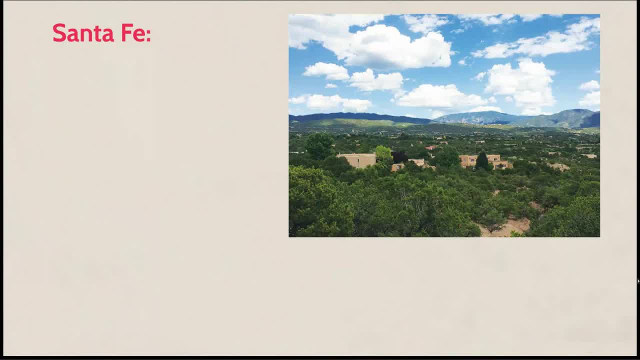 narrowed landscape is surrounded by a chaperon, so to placing it in a very highly prone area to wildfire. and what they've done is they've applied an overlay district and an overlay district to assess standards within a very specific zone or boundary, and those standards supersede all existing. 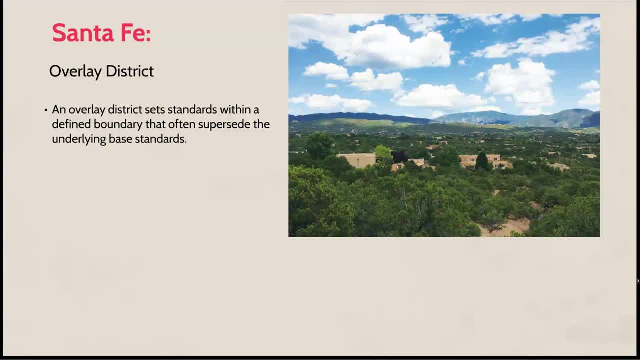 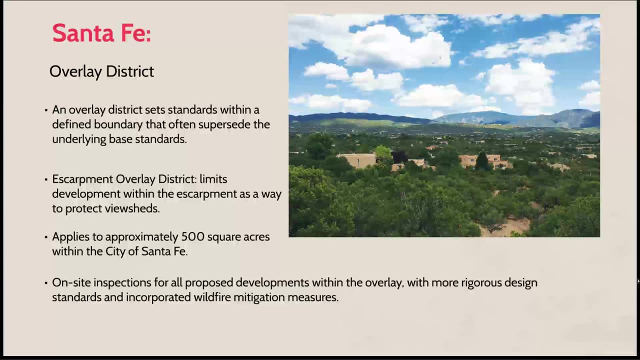 regulations that might come before it, but actually it takes hierarchy. it's a falls within that specific overlay district And what this was originally passed for was to protect view sheds that were situated within this escarpment, And this escarpment is about 500 square acres that surrounds the city of Santa Fe. 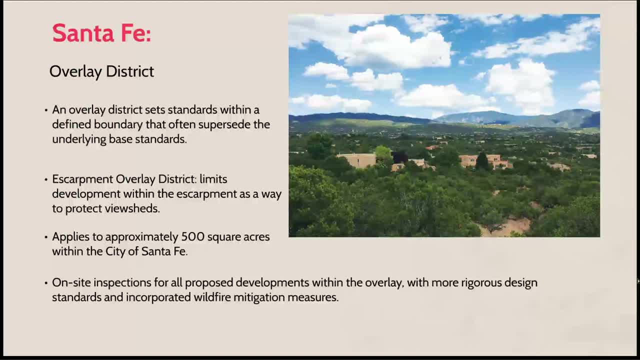 It's where the chaperone kind of meets the foothills of the surrounding mountains And it's prized because it is such a gorgeous area and because of those view sheds and what that might appear like on the horizon line. So I think this is unique in that Santa Fe has applied an overlay district within the 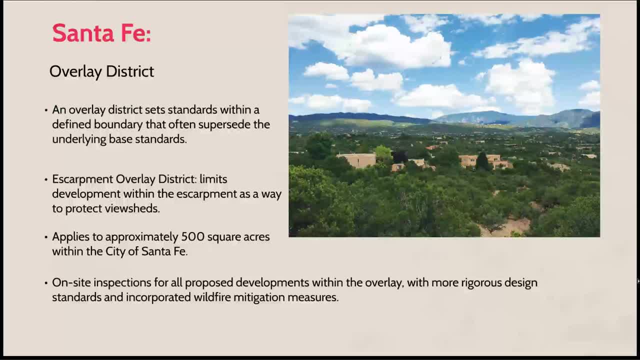 escarpment area, Again originally intended to protect view sheds, but in doing so they've applied fairly stringent development protocols within this area. that also couples with wildfire risk reduction. So, for example, any proposed development within the escarpment overlay district has to be: 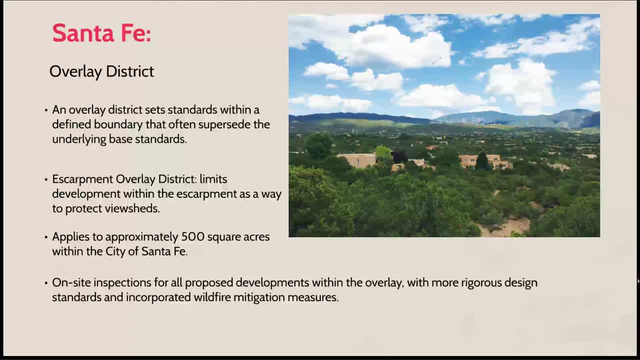 inspected not only by the city but an actual on-site mitigation process, And so it's just a way for them to apply another set of standards and regulations regarding how that home has to be developed in order to incorporate wildfire mitigation into the escarpment area. 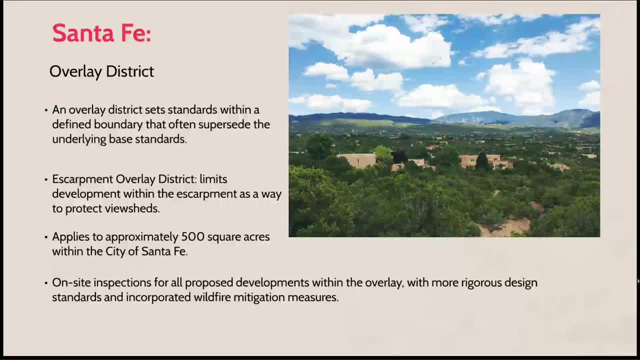 And that's kind of where we're at with this, And I would say that, again, we're doing a lot of work and we're working on what we're doing into its actual design. so this is how santa fe's approach. wildfire risk, again, not initially. 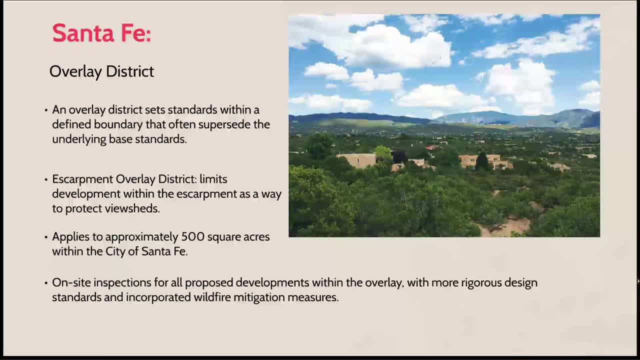 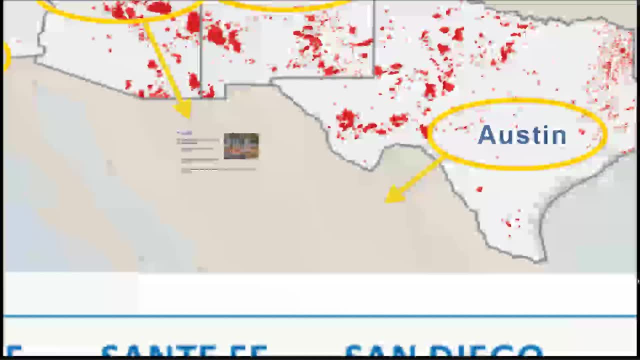 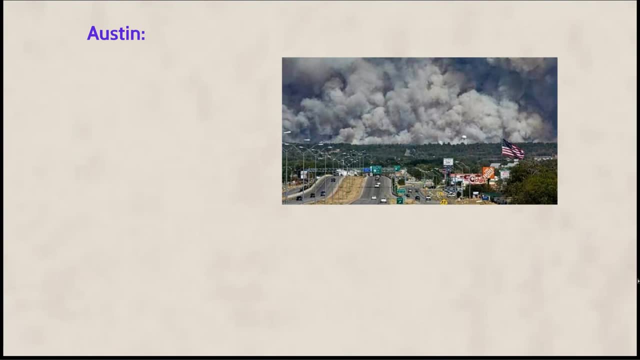 intended just for wildfire, but also other conservation purposes within that city's boundary. um looking at how austin has done it: often- and we all know if you've been to texas- they're not big proponents of land use regulation, but what they've done is, as one of the fastest growing 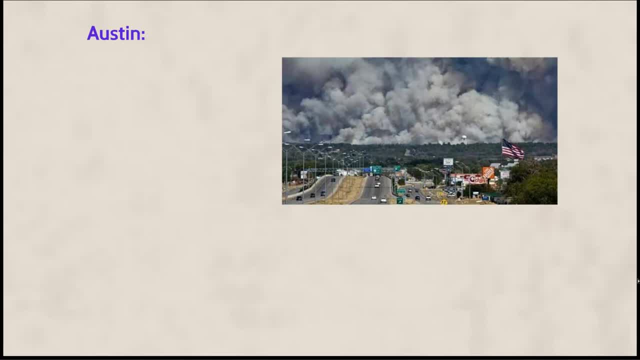 cities in the country- not just the west, but the entire country- often has anticipated ongoing growth within the wui, and so what they do is they work very, very closely between the city and then travis county, and so it's a very multi-jurisdictional collaboration between 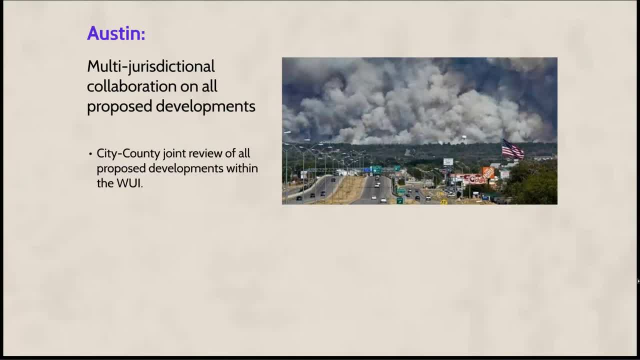 the two bodies, and so they actually have a joint review process of all proposed developments situated within the wui that abuts both the city and the county boundaries, and in doing so, they're going to be able to do a joint review of all the proposed developments within the wui that. 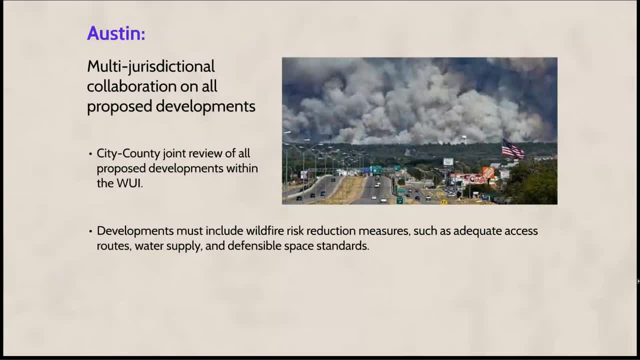 abuts both the city and the county boundaries, and in doing so they're going to have a joint review. they require an additional set of risk reduction measures that might only you know, be applied to just the city. now the county is requiring it as well, so it's a double um, a double layer really. 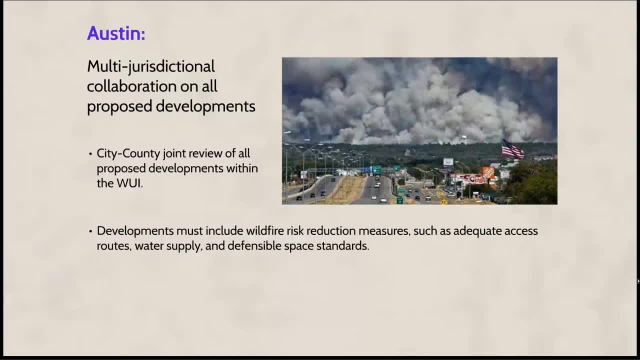 of how any developer can um design it and construct homes within this area, again fairly similar to flagstaff in that some of it requires hardening materials if necessary, but certainly other issues such as adequate access routes, water supply, defensible basement standards and other things that are requiring homeowners to have these mitigation measures in place prior to. 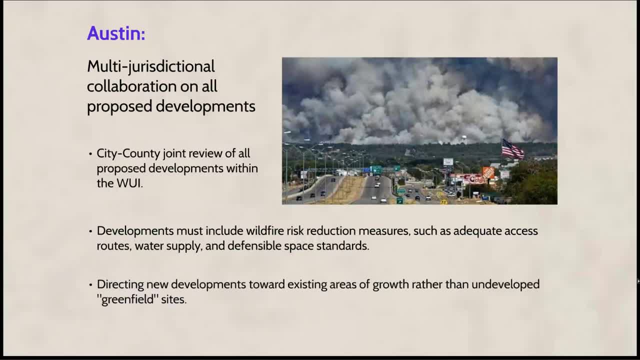 actually developing or living in any of those areas. they also are really active about trying to encourage development away from the wui in general and more towards brownfield areas rather than these greenfield sites of undeveloped landscapes. so this is how austin has approached it. 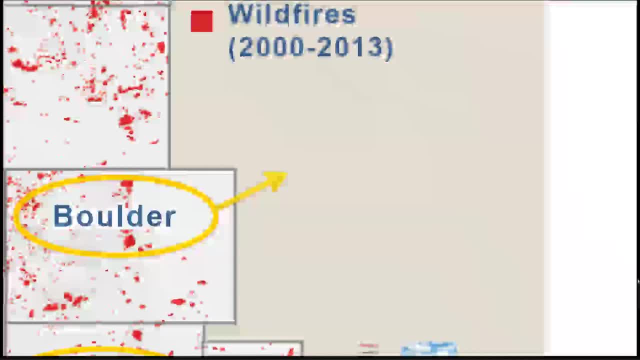 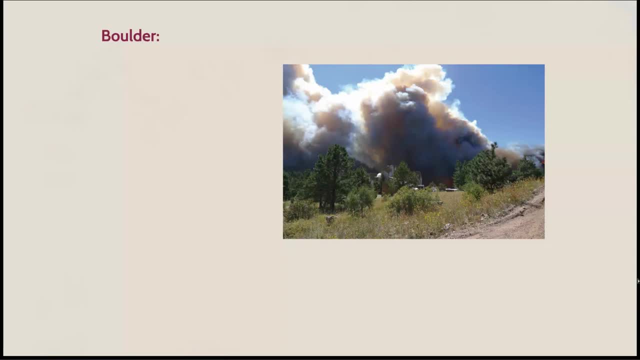 and then looking at what boulder has done. boulder, if you've been in that area driving up to boulder, a lot of the lands immediate to the city have been protected under an open space conservation easement. uh, not so much specifically again for wildfire risk, mostly for other conservation and 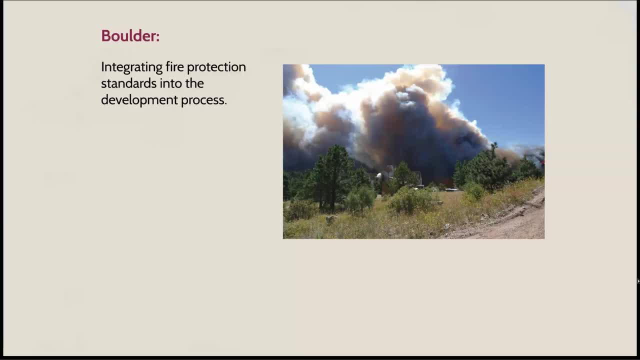 open space purposes, but in doing so, they've also provided a buffer in that region. they also require hardening materials as part of the actual land use code. and then something that's really unique about boulder that's really quite creative, is that they have this public-private partnership. that's 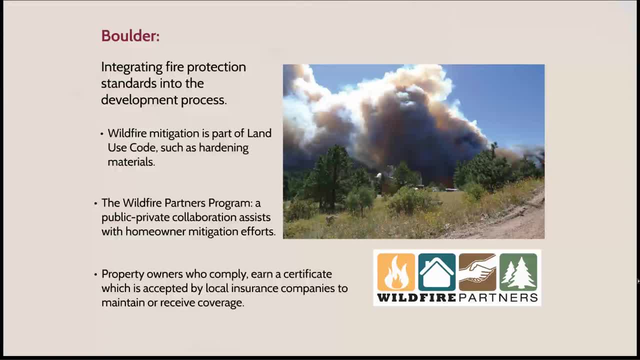 called the wildfire partners program, and this is when a private homeowner situated in a high-risk area can become part of this program and an actual mitigation specialist comes to their home site and works with that homeowner over the course of a full year to integrate defensible space standards. 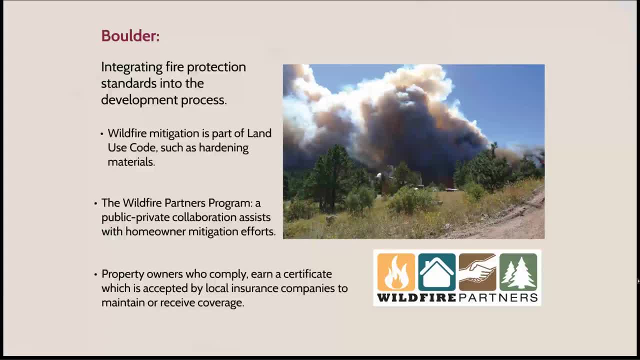 or are certain hardening materials or other mechanisms that are on a site-by-site basis to reduce wildfire risk within that property, and so, over the course of the year, the mitigation specialist works very closely with the homeowner, and then the homeowner in turn can take this certification, after the one-year process, to their insurance. 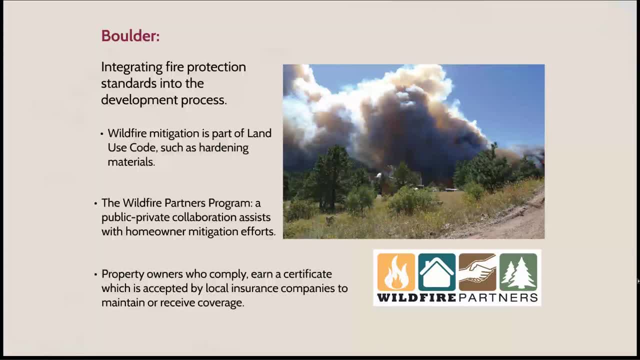 company to apply for either ongoing coverage or certain benefits within their premium. and really what this program has been really great about doing is acting as a public awareness program, in that one homeowner you know gets a certificate and they get a little sign that they can post in front of their house and they are encouraging their neighbors to apply similar. 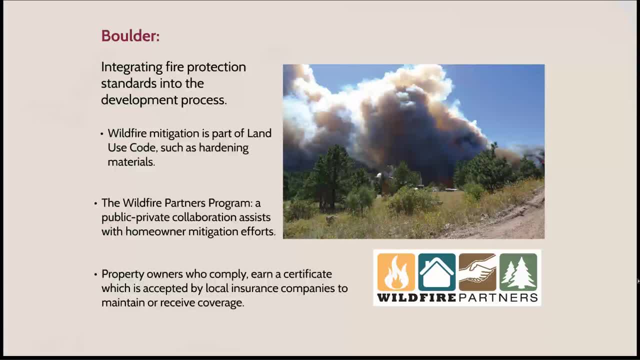 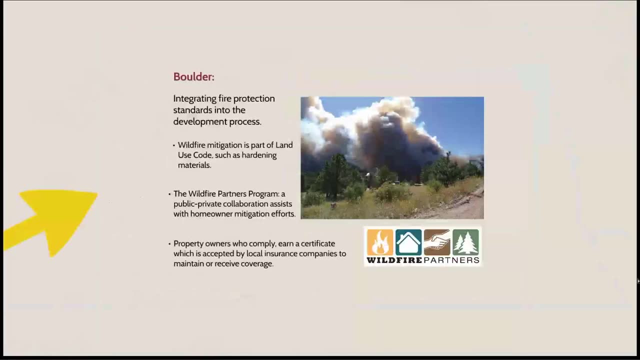 measures within their home. so then the neighborhood as a whole can be recognized as a participant with a wildfire partners program. so this is a really innovative, again fairly progressive, way of being able to deal with wildfire risk within the city boundaries. so those are just a number of the key examples. we have a whole suite of different measures that were profiled into the. 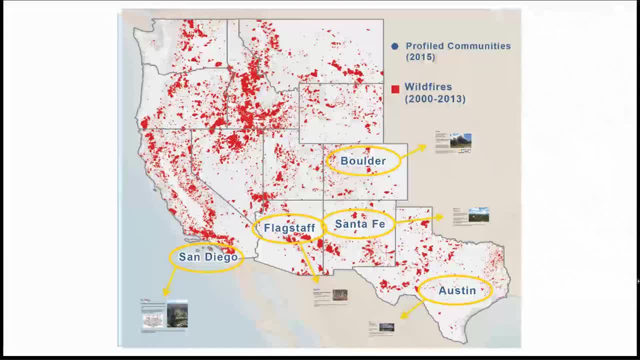 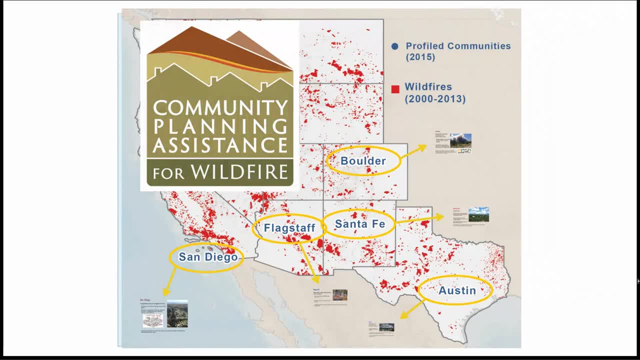 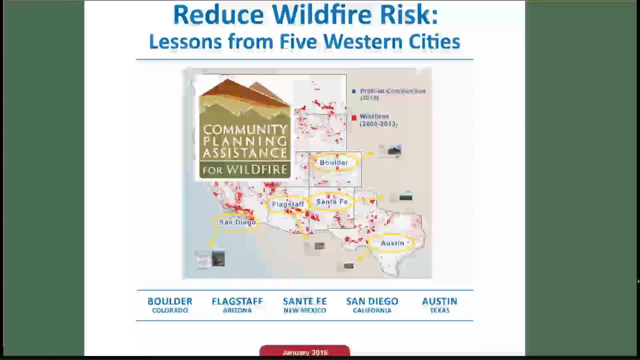 full report, but i just wanted to highlight the top ones that stood out as being some of the more unique examples. again, this is all encompassed within this larger program that headwaters economics has launched- that's called the community planning assistance for wildfire program, and what this program does. 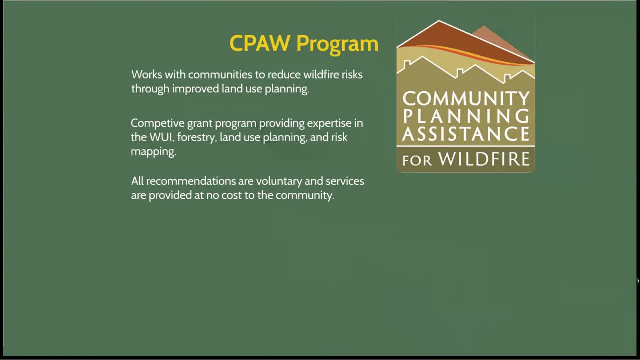 is. it provides communities with free consulting advice in the form of either land use planning or forestry expertise or wildfire risk modeling efforts to better understand where risk is highest within their community and then how they can work to integrate that risk into how they plan to develop and manage their community. 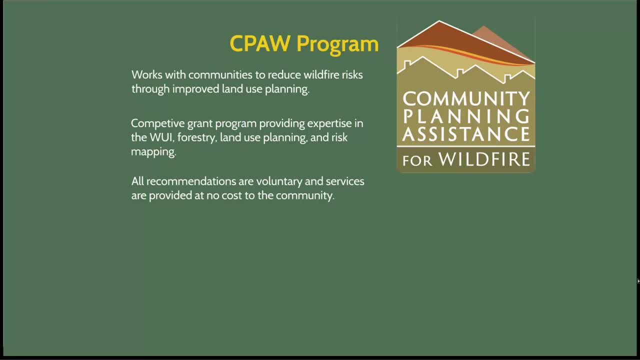 and move forward within their community strategies, looking both in the short and long-term future. it is a competitive grant program and, again, it's providing expertise within these specific arenas and all recommendations are voluntary. there's no obligation to becoming part of the cpa program other than having the community capacity and political will to support whatever. 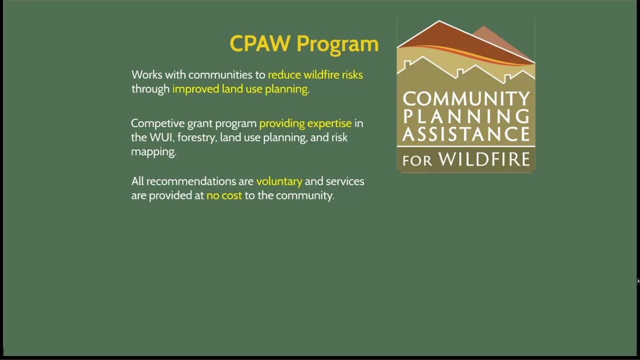 recommendations come out of it, but again, it is voluntary. we have no obligation to the board of commissioners or others to make sure that they are actually put into practice. um and again, everything comes at no cost to the community. these are free services. some of the examples that have come out of it, as i've already discussed, look at things from: 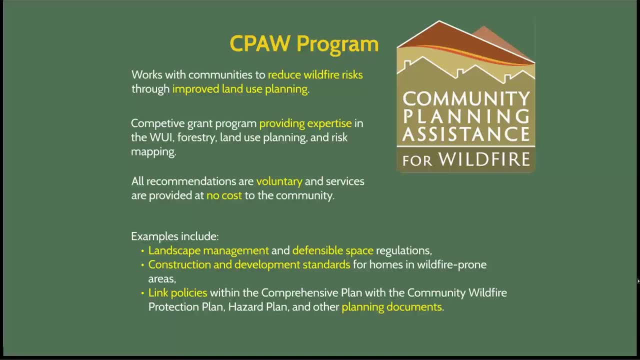 land management, dispensable space regulations to actual health subdivisions and proposed developments or design and then linking policies. and this one is more of a actual marrying process where we try to integrate the comprehensive plan and the growth development plan with things that are already stipulated within the community wildfire protection plan or the hazard. 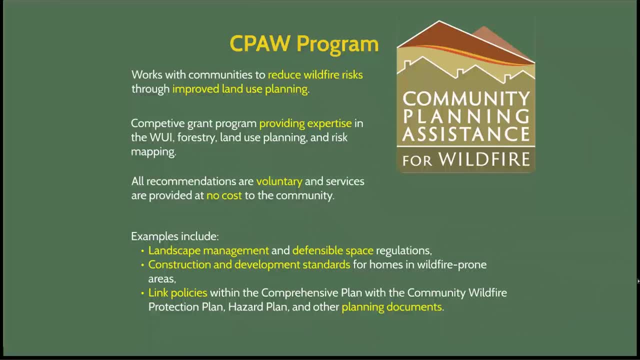 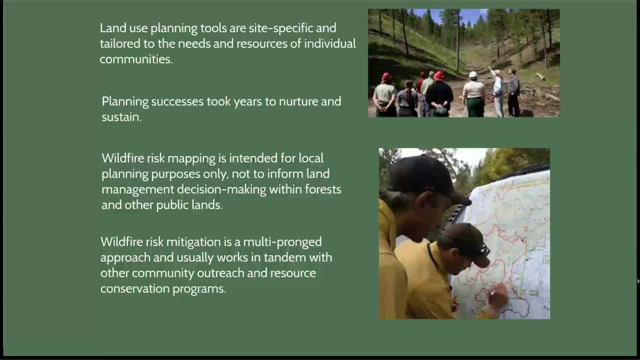 plan and other and other documents that they actually reflect and can be coupled together in a way that speak to one another more so than are often done uh in in most areas. so that's the overall cpa program, some of the things that uh come to note and that we learned over the course. 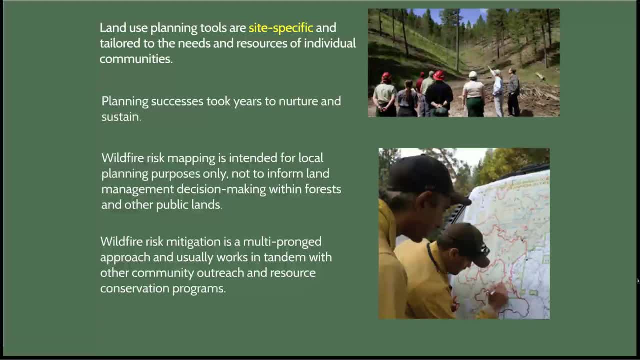 of this past year is that these land use planning tools are very site specific, so they're customized to fit local context and in that way they're very much tailored towards the needs and the resources of very individual communities. and so, while there might be this- you know- arsenal of land use planning, 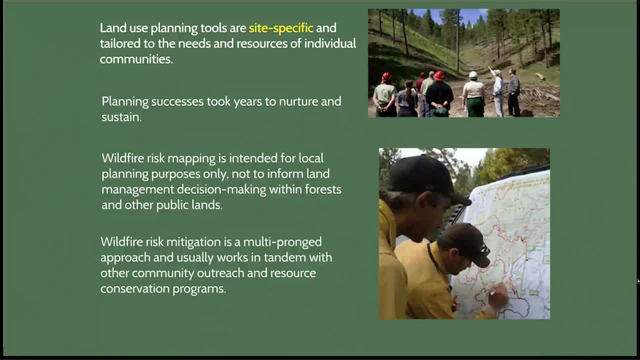 tools out there. in reality, maybe only two, three or four of them are going to be applicable to each community um. the planning successes within these communities, particularly the collaborative partnerships, took years to nurture and sustain a lot of relationship building um and with time we're very successful. but it really required commitment from the very beginning and early on um and that 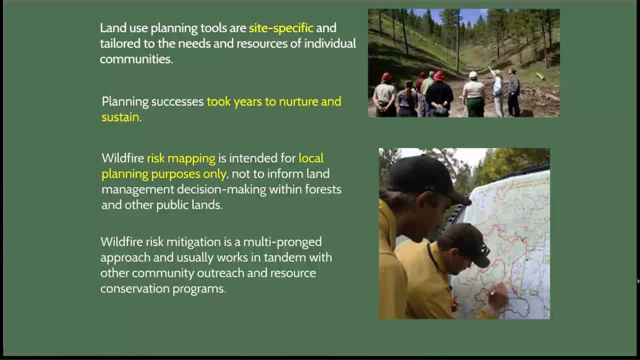 some of the wildfire risk mapping efforts that we provided for the communities that really tended to focus specifically on just the community level and their planning purposes for wildfire risk. they're not intended to promote management within the larger forest or public land. that's not what it's oriented to. again, we work with the community on a one-on-one basis. um, and then wildfire risk. 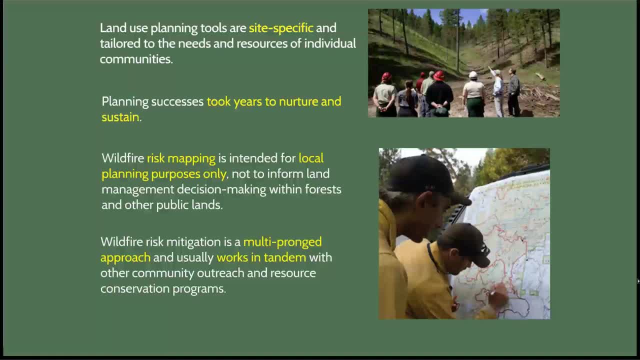 general is very multi-pronged and has to work in tandem with other conservation and research efforts. for example, protection of watersheds or open space policies can often serve as the umbrella or couch larger issues about wildfire risk, and so that's something that we're certainly 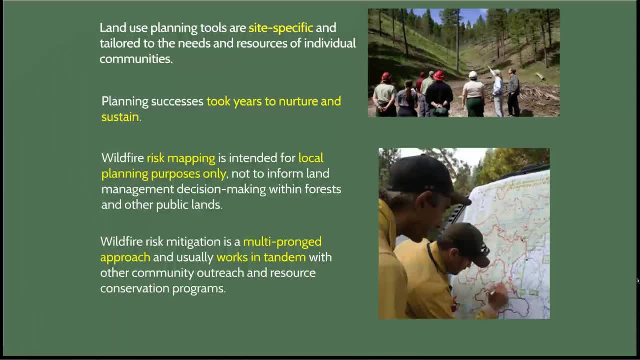 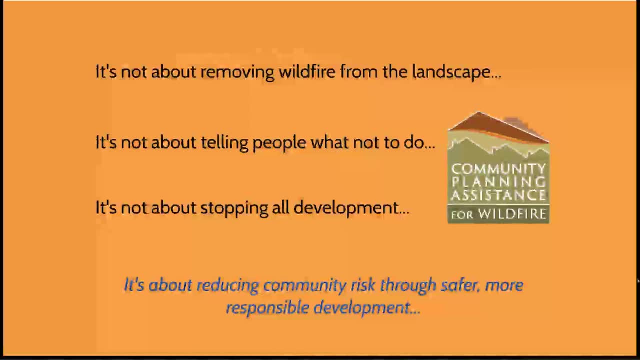 learning as we move forward is how much these two can all work on, you know, alongside one another. um, um. what this program is focused about it's really not looking at how we can remove wildfires from the landscape. we, as scientists, all recognize that that's an intimate part of an inherent part of 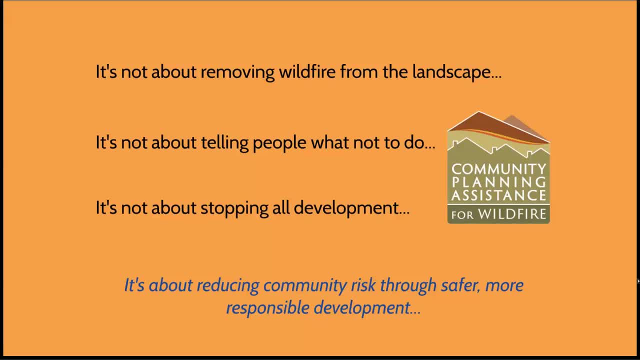 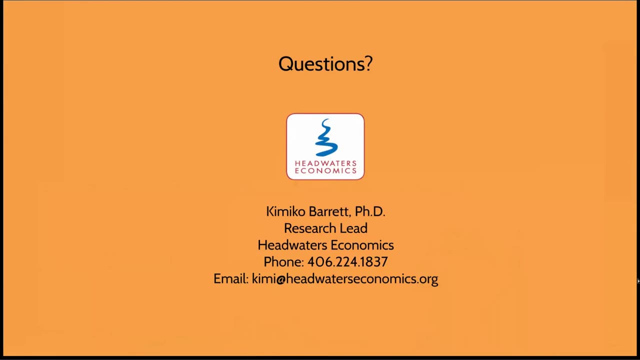 creating a healthy landscape. it's not about telling people what they cannot do and it's not about stopping all development. it's really trying to promote safer, more responsible development in those places that are already set up for ongoing growth. um, that's really all i have. um it's. 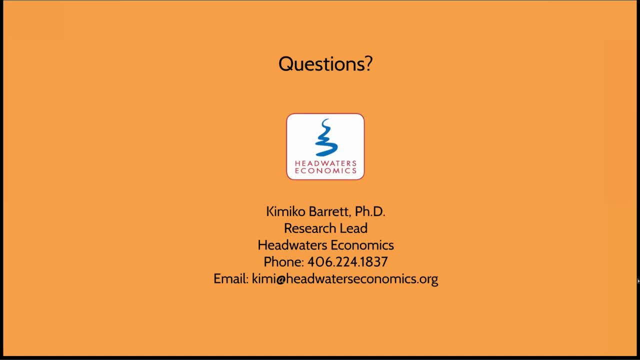 i tried to keep it to about a 30 minute presentation or so, um, but i'm certainly willing to answer any questions at this time, um, and turn it back over to stacy. uh, here's my contact information, so i welcome any feedback or if anybody wants to know more about some of the 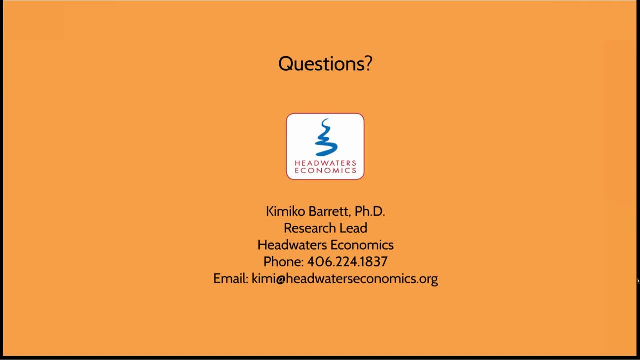 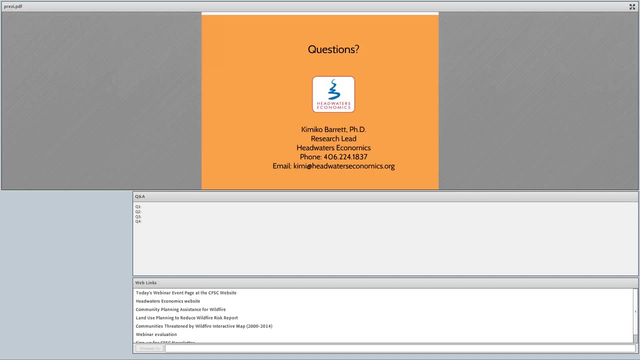 other research we're doing. please feel free to reach me, okay, great, so i'm going to switch screens real quick here so we do have plenty of time for questions, um, and so i'm going to give you guys a chance to type some questions in the chat box there, and while we do that, 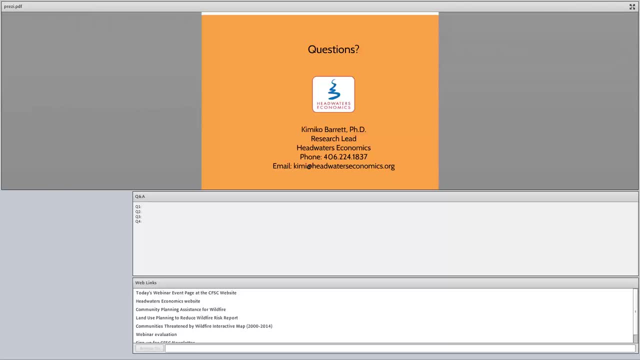 i'll take a minute here and go over some of our links. um, and so her contact information is right there too, if you need to make note of that. um, so today's webinar event page at the at our the california fire science consortium's website, and so when i have the links of this recording up, i'll 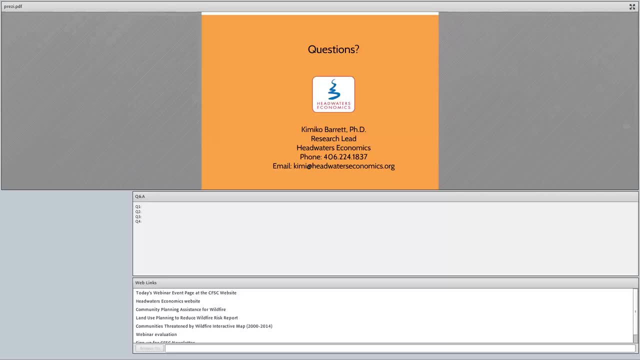 put it there, and any of these resources and website links i'll also add to that website. so that's a good starting place. if you, you know, just need to get more information from today's website or a webinar, and then it looks like: actually, kimi, do you want to go over the next few, since you added? 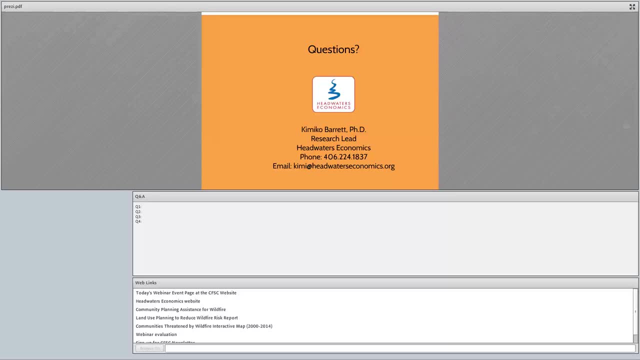 the, the websites and such for the web links at the bottom here. yeah, absolutely, um. so let's see here. as i said, i work with the group headwaters economics. we do a whole bunch of different research on the west. we are all researched. there's a staff of 10 of us. we are research. 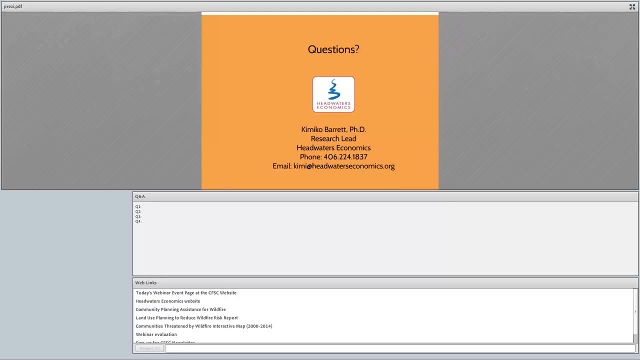 analysts and data geeks. so the wildfire program is something that we've delved into the past couple of years, but ultimately the sepaw program is going to be turned over as a loan nonprofit and headwaters economics is going to step back. we've been incubating it for the past. couple of years and we work very closely with a wildfire planting planning international and a gal named molly maury. there she's our partner and effectively she will become the new executive director of the seapaw program and headwaters economics is going to go back to doing what we 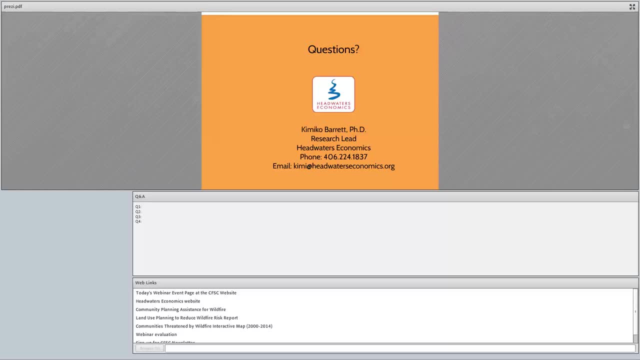 do best, which is mostly research on other issues in the west. so i've set that link up as well as a community planning assistance for wildfire. again, the CPAP program link is there. there's more information about some of the communities we've worked with, as well as ensure materials about how interested communities can apply. looking 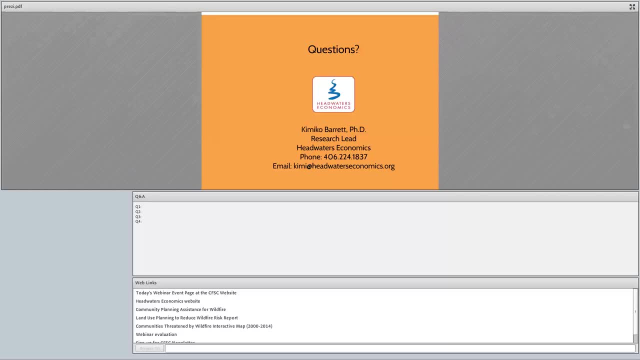 at the. this is the actual report. the land use planning to reduce wildfire risk is the actual document. that was the deliverable of that initial profile study and then I have a link up there. we do a lot of data, viz, visualizations and interactive on our website- different ways of looking and seeing different. 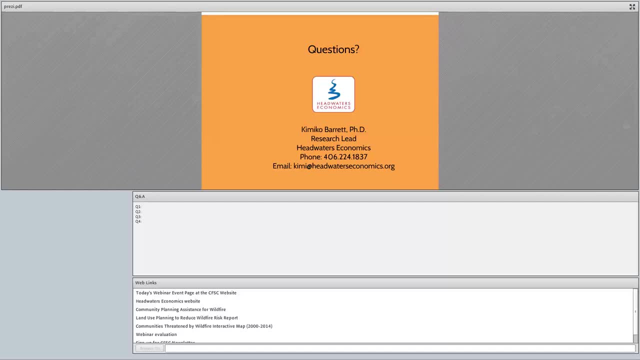 studies or different information on topics that face the West, and so one of them was looking at what is the historic patterns of communities from the year 2000 through 2014 that are most impacted by wildfire occurrences, and so that's an interactive map that allows you to see that. so again we've got. I would invite. 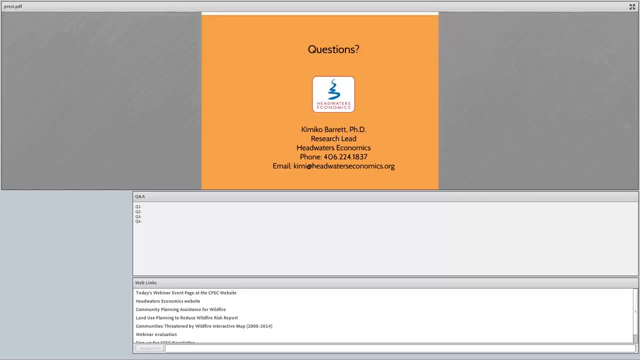 you to go explore some of those data visualizations. there's everything from economic profiles looking at what communities are most at risk in the West and really throughout the country, but lots of valuable information for those who are involved with this kind of field and scientific arenas. so, yeah, those are the website links I've listed. Stacey great. 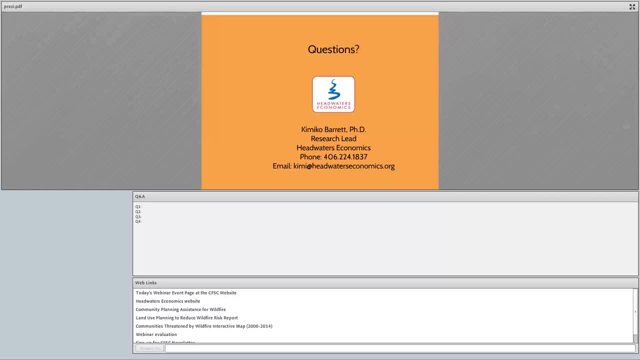 thank you, you did a much better job of that than I would have the last two links. there's the webinar evaluation, so when you exit this room you'll be directed directly to a short evaluation. it's just a couple questions, should take you a couple minutes, and it really does help us at my organization. both know that this is. 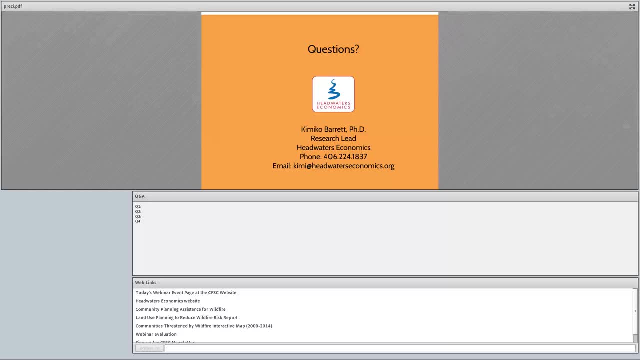 useful, improve on future webinars and also to report back to our funding organization. and if you type something in about future webinars, we've actually done webinars. we do use that feedback specifically to try and tailor to our audiences needs. and then the last one, if you're not already signed up for our 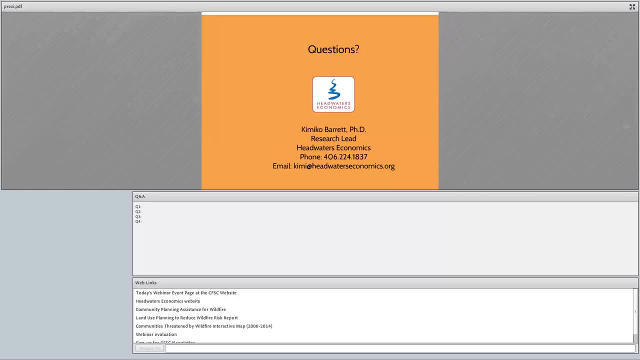 newsletter. it comes out once a month and it talks about upcoming webinars, field trips and new research briefs or other products that we have out. so you can click on that link and it will direct you, if you get browse, to lead you to a place where you can sign up for that newsletter. so that's most of my. 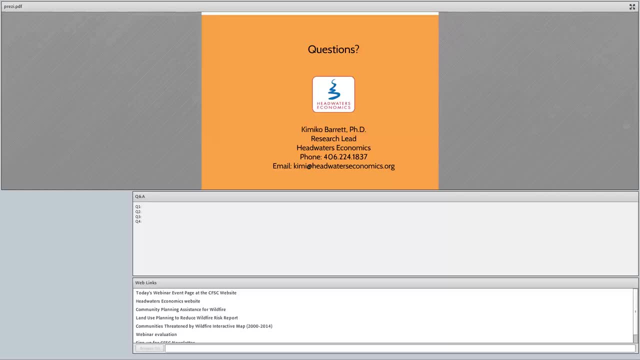 housekeeping things and we do have some questions, so I'm just going to put them in here and go through them. the first question was mentioned earlier on, before. you talked about San Diego, but is there any future plans to test further in California? absolutely, it's something we've been pushing on for quite a while. 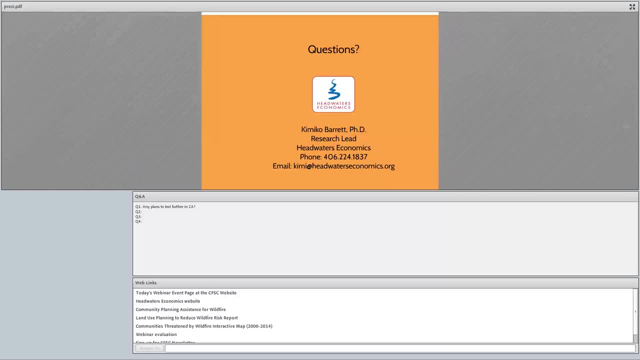 at this point, the one thing with with California, obviously, that there's Cal Fire, which is such an amazing asset in that area and they such a quiver of resources already at their disposal that it's something that we would want to approach in a way that we could work with Cal Fire and make sure we're not 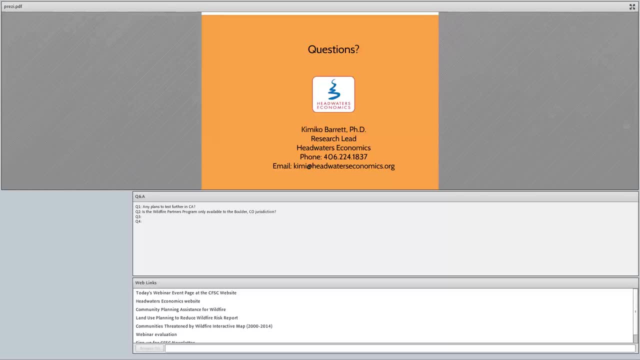 trading on any toes and and really with having the utmost respect for that program, we just want to be tentative approaching how we would work in California. but yeah, absolutely, given their their class, fire risk and and their history, I don't think we could continue with the program without. 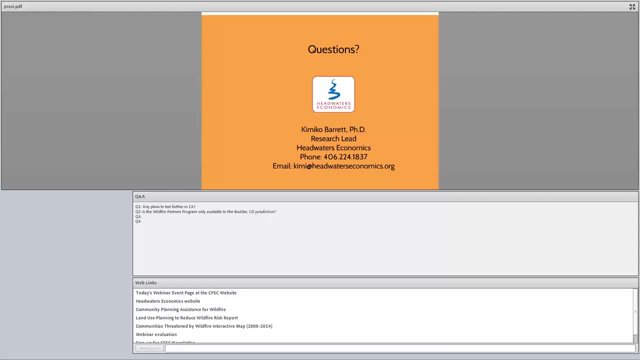 involving a California program. so it's something that I, as one of the program managers, has been pushing for for a long time. so it depends if a community from California applies, that's. the other thing is they have to express interest in actually wanting to participate in the program before we just you know. 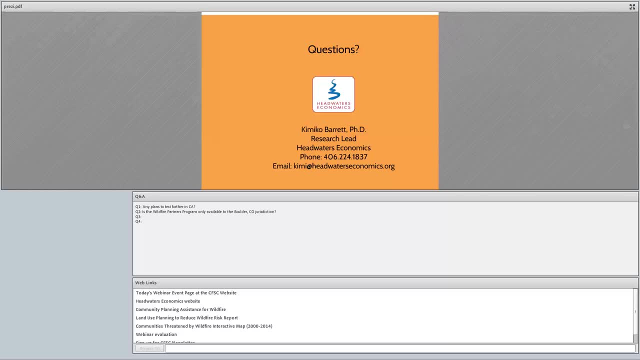 solicit it from them. so yeah, that would be the answer to that. so yeah, I guess the next question is a wildfire partnership program only in California. is there any available in Boulder, Colorado? yes, I believe so, because it was kind of a homegrown program. it came out of very innovative thinking from those folks. 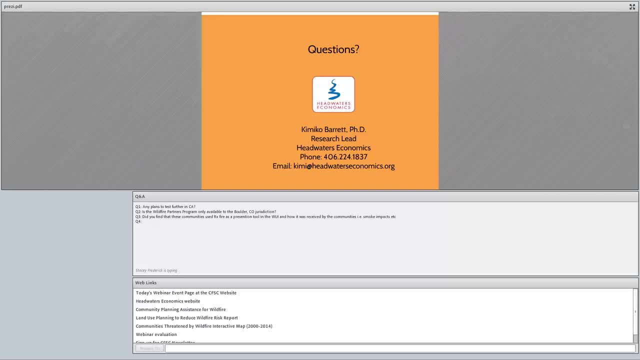 that deal with fire there the most. so yeah, it was. it's a really awesome program. it's still in initial stages of really trying to expand into into a broader jurisdictional program, and so I can think they're still experimenting with how that can be best implemented. but the 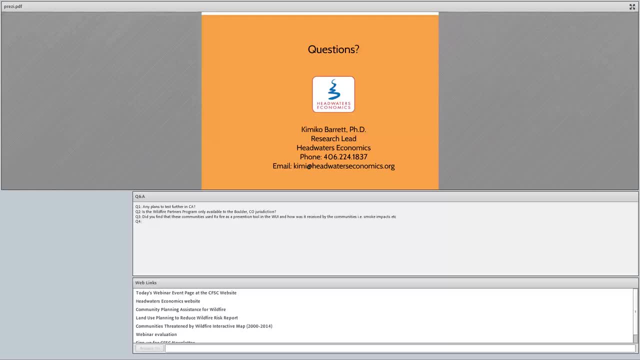 guy that that works with it, Jen Webster, and in Boulder, Colorado, very good resource for that. so yeah, that's the answer. that question is: I do believe it's only available within Boulder. did you find that these communities use our expires prevention, and by RF I'm assuming you mean prescribed fire, if 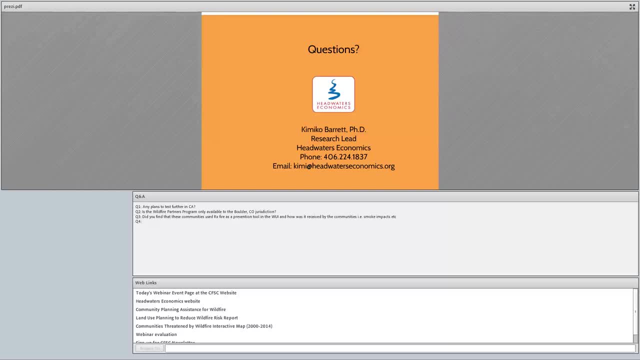 there's another. I'm sure that's what that is, yeah, okay, yeah, I'm sorry that wildfire science is still not my area of expertise. that's why we contract this work through wildfire planning international. but it was so. Lucy, did you find a community? so flat staff was really one of the only. 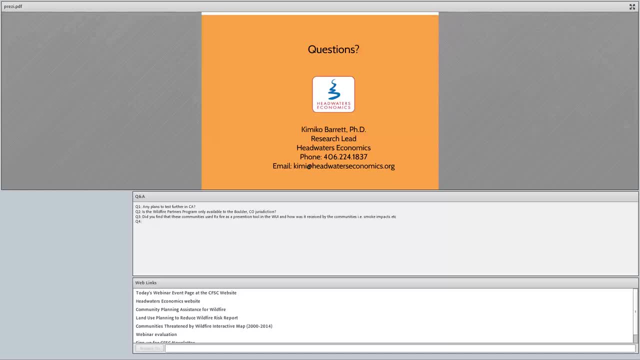 cities that actively used prescribed fire as a mitigation tool and in terms of the city that we profiled, I'm sure it has been demonstrated in other areas, but Flagstaff was the one that stood out the most with that and it was received well by the state, the community, because 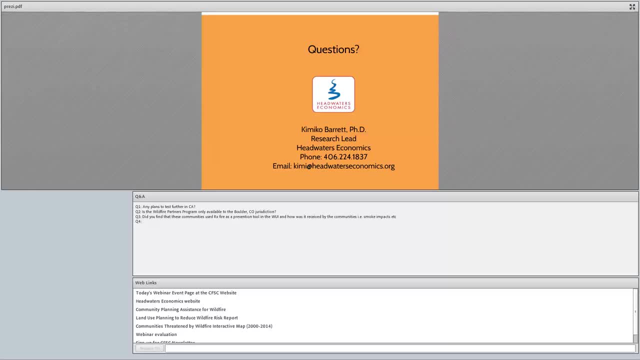 they're the ones who passed it in their bond measures and really what happened is that the community leaders galvanized around the post wildfire impact in 2012 and used that as a trigger event to get that bond measure pass. I don't think it would have been so successful had it not been for the fire action that we've been. 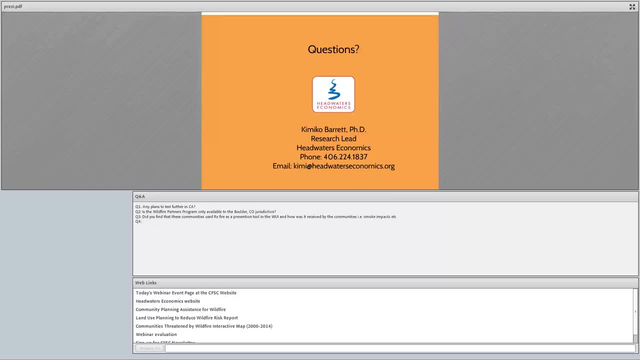 working on, and so I think that's one of the things that's really important to think about is that the community was able to accept the smoke as part of the aftermath, and knowing that, in turn, they were reducing wildfire risk not only within the city itself, but there's no watershed above, which is so valuable, for 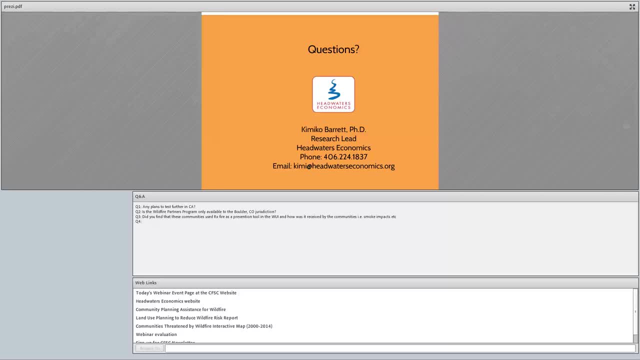 that community. so that's really one of the only areas I've seen where it's been very, you know, used to the debris that's in the community, and so I think that's one of the things that's really important to think about. is that the how it's done in terms of, you know, the the community in terms of it's been? 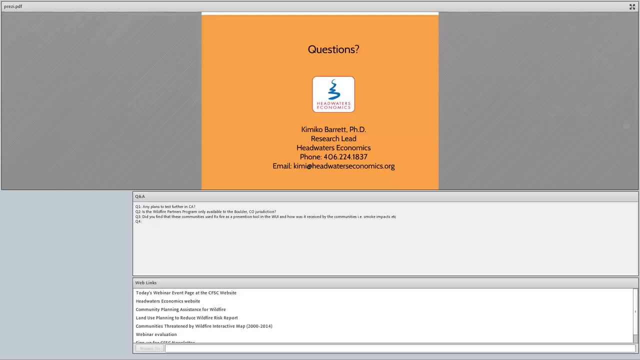 received well and also on the city, can understand how much it was burning and it was getting fire. the fire was getting caught on fire and it ended up hurting the city. I think it was a pretty big thing. it was a huge story and you know, sometimes you don't know how bad it was, but it was a really huge thing when you 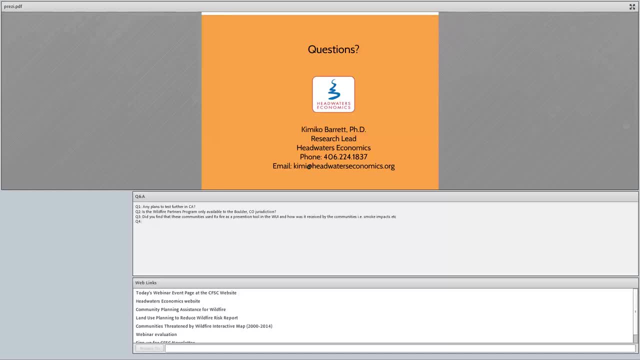 think about it. so I just want to say that I definitely think that it was a huge thing and that's why that it's so important that it was. it was a huge one of the many times I played and it was just so big and it seemed like it would. 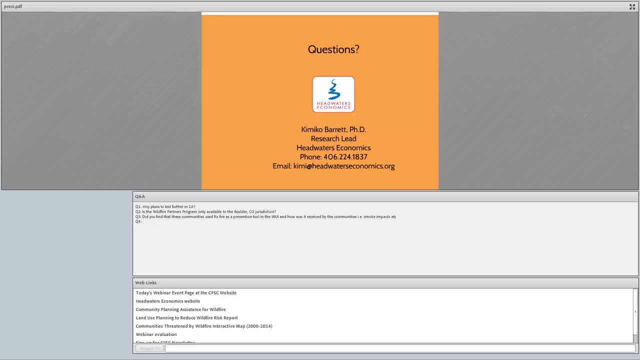 be the highest thing that any of you have ever experienced with that sort of fire in the city and it's definitely a huge thing because it's not just two, one of the many times I played and it's definitely a huge thing because it was of people come in there. you know, small communities, small firewise groups wanted. 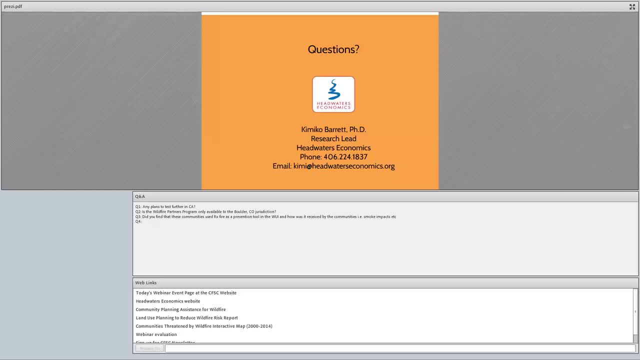 to prescribe burning, but they don't have the expertise or the tools. so, with this one in Flagstaff, how exactly was implemented was it? do you know that or I? I don't know how it's exactly implemented. I know that they work very, very closely with Forest Service to do it and I- only I, the gentleman's name. 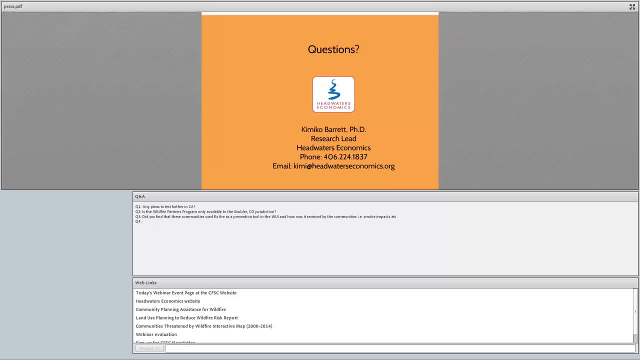 that was part of that. Paul Somersfield is a great resource down there, but I don't know the actual steps and strategies beyond. I know that they established a separate program. there was a private public partnership called the greater Flagstaff fire partnership, I believe GFS- key with the acronym- and so 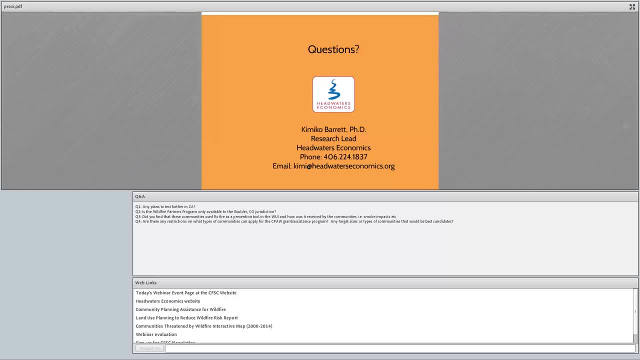 under that umbrella kind of that larger body that was both high public and private entities, they were able to push for fuel treatment programs within the city, and so that's what they were able to do, and so that's what they were able to do. so I think, using that, it was a very collaborative, multi-scalar partnership. 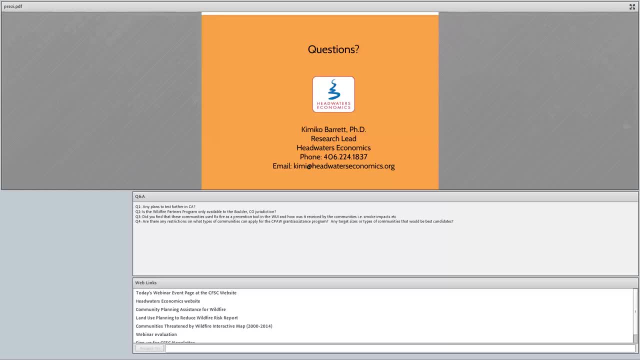 that literally had partnership in its name was a good way to be the messenger and kind of the vehicle for any sort of fuel treatment work. and so you know, I think involving local community residents as well as agencies and city leaders works to be the catalyst for that kind of treatment in the city that. 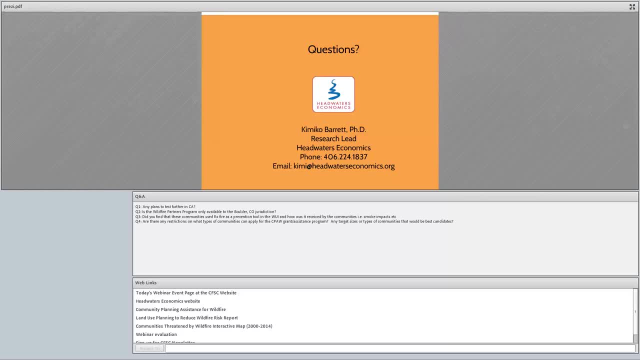 answer your question, Stacy. yeah, that was great. thank you and it you know I'm getting a lot of questions and about this program, so there's absolutely interest, so we'll keep going. since we do have time, I'll just read question for you. go ahead. I was just going to say there's we have. 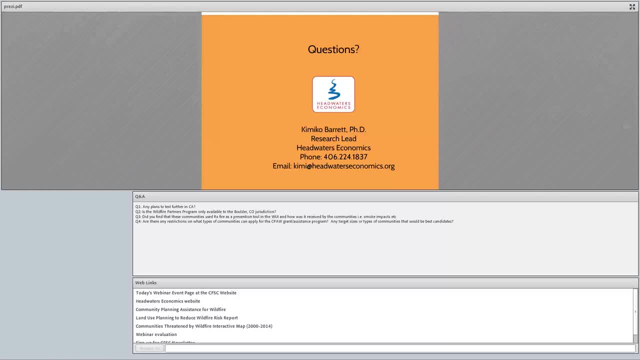 contacts on that land use planning to reduce wildfire risk report. there's actual contact names behind each of these cities and they're- you know those guys. I know they're all in their fire season right now, but they're also really great individuals with a lot of knowledge about each of these specific. 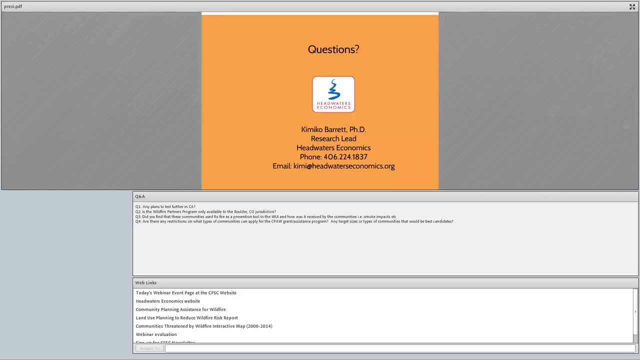 tools. so I would recommend that you go to their website and find out more about each of these specific tools. so I would recommend that you know trying to reach out to them or their departments if you want more detail. and then, yes, I'll just jump into question four. I see that. are there any? 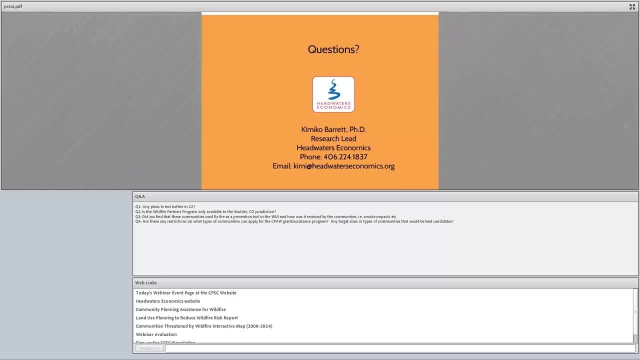 restrictions with types of communities that apply there really is not with respect to scale or jurisdiction size. we're working, you know, with the entire county of health and then just the city of Missoula, so it's very different in each area. what we are wanting to ensure is that the community or the county, or 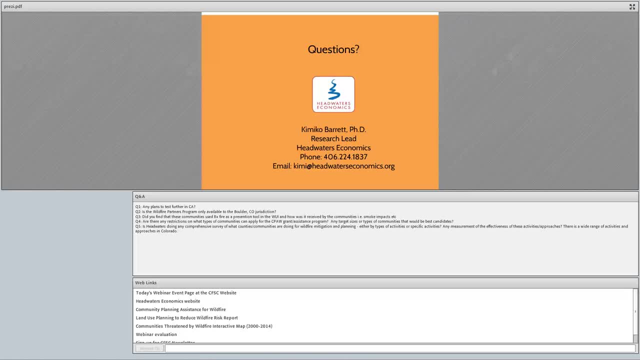 whoever that body is that we work with actually has the capacity and the willingness to work with us, because it requires, while not any financial upfront cost, it requires time and it requires commitment to meet with us. we were in town. schedule appointments, if we ask for it, so that some of the modeling results, and it's a 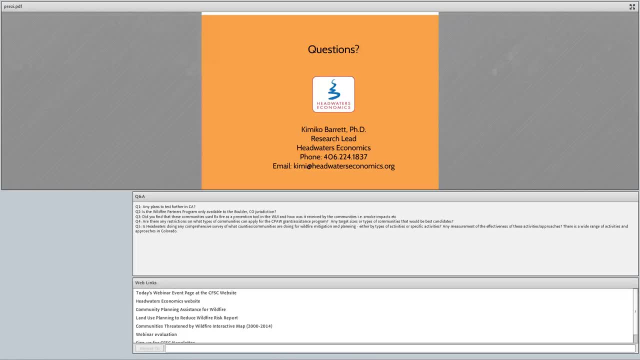 fairly intimate process, and so we really need to see that this is something the community wants and that they're willing to continue with our correspondence with us to ensure that what we suggest can actually be implemented. so we don't want to just kind of be a place holding program. we really actually want to put 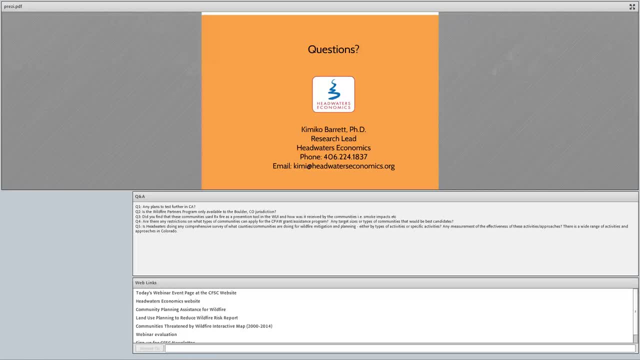 this practice into into reality and on the ground. so yeah, there really is no restriction in that manner, so I'll go on to question four: is headwaters doing any comprehensive survey of what counties, communities are doing for wildfire mitigation and planning any measurement of the effectiveness of these approaches? 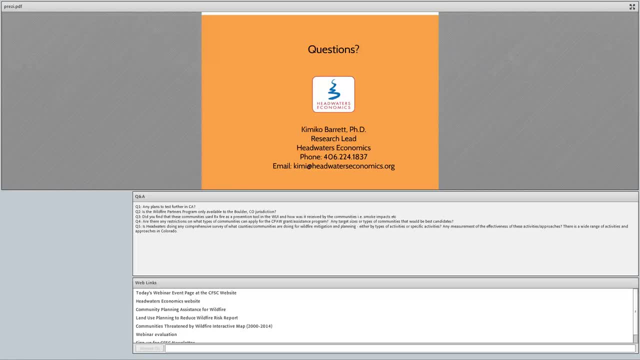 that's a great, great question and right now you know we're not doing a comprehensive survey- could say, really, what we've done has been this profiled assessment of cities and we chose cities because we figure if anybody in the West is going to be doing really aggressive tactics to reduce wildfire risk, it's. 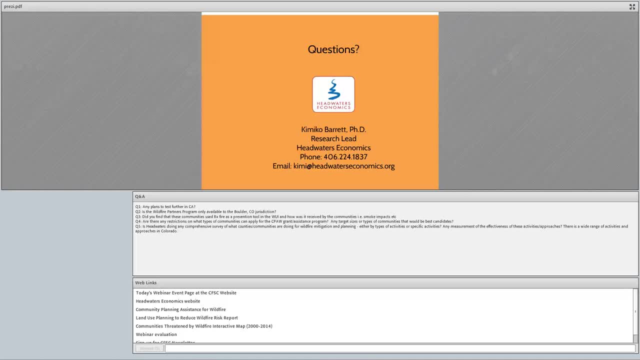 going to come from a city that's got the resources and the capacity to do that. so in terms of kind of a wider blanketed survey of all scales and counties, communities across the 11 the western states, we have not done anything like that yet, particularly given the qualitative nature of it. we're a bit more data analytically driven, so 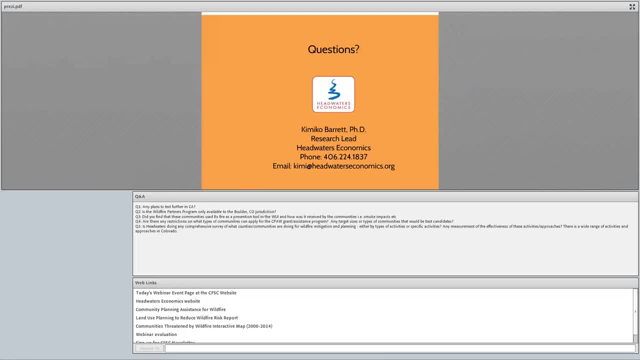 we would almost need to have almost quantitative measurements of something like that to be able to implement that kind of study. but I also find it incredibly fascinating, so the effectiveness of being able to actually apply metrics to the success of some of these approaches. you know that's a. 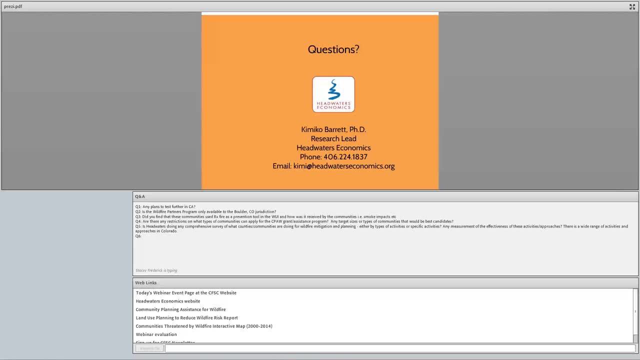 hard part right. is that a fire, you know? does it really strike the same place twice? and then, what kind of time period is it coming through? a community makes it really hard to measure how successful something is, so we're hoping to apply that kind of metric to. yeah, I see that's the next question here. what's the? 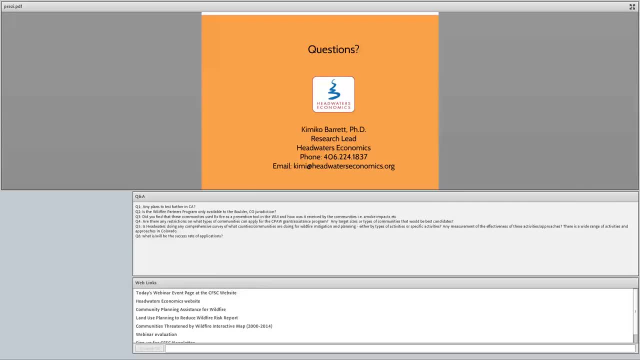 success rate of the application. so what we're doing now is: please note that this program was just launched in 2015, so fairly new. so what we're going to do is we're going to think about what is the success rate of the applications. so what we're doing now is: just please know that this program was just launched in 2015, so fairly new. so what we're doing now is to 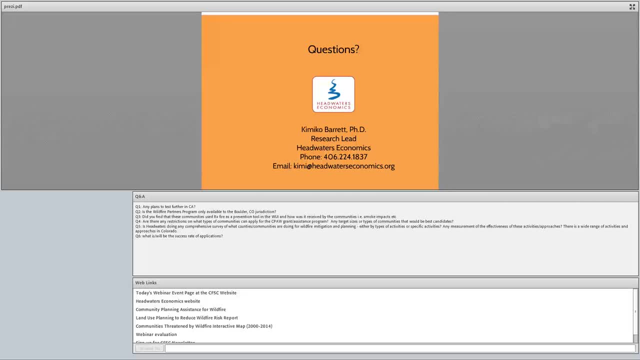 What we're doing is, before any work is done in these communities, we go in as a team and assess it and work with the planning documents already in place and talk with the foresters and the Louis specialists and the local expertise of fire knowledge in those areas. 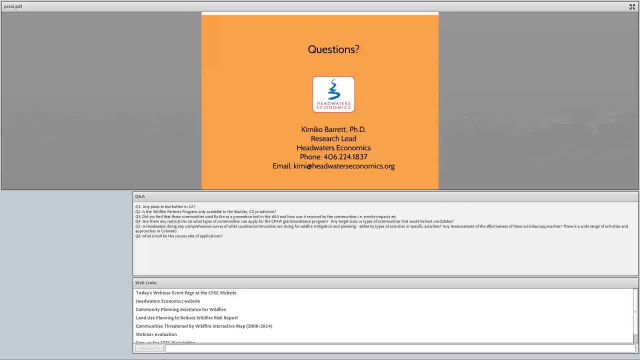 We do a pre-CPAP program rating and measure a couple of different areas and components of land use planning to see how well they integrate wildfire risk And then after the one-year program we apply the same rating system to see, given the implementation. 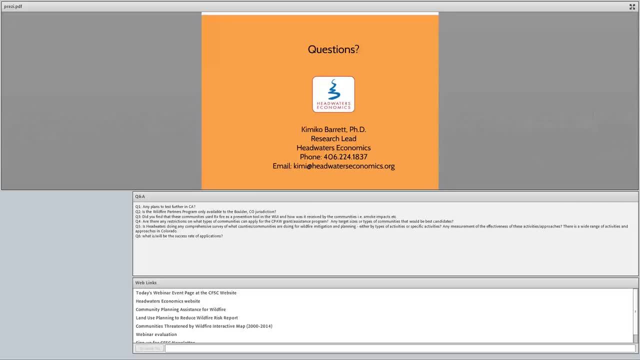 of some of these recommendations. has it worked? Again, that's hard to say until a wildfire comes through the area. So somewhat of a moving target, but we certainly want to be able to apply a metric to understand success rate better. That would help us in every way, particularly given that we are very data analytically driven. 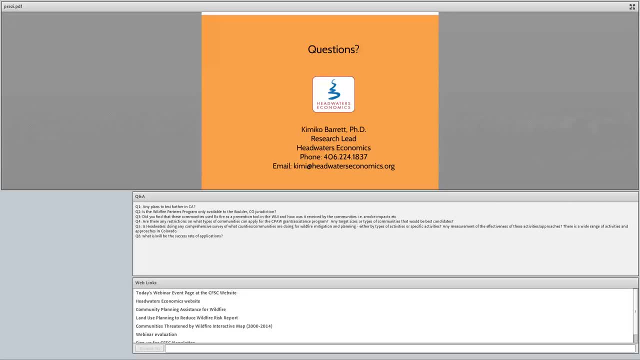 so we're trying to reach that. But if you have other thoughts, I certainly welcome other ideas about how success could be better measured. That's one of the things that's difficult about a program like this and the nature of wildfire in general. So it looks like that's the final question. 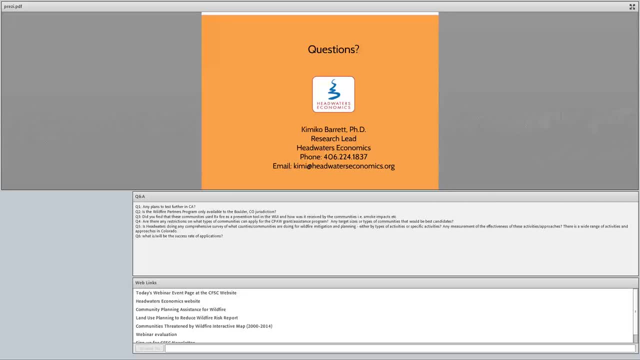 I would open it up to anything else here in the remaining minutes, unless Stacy has some follow-up information she wants to send out there. No, I think that was great And there's, like you said, a couple more minutes, so if anybody has any last-minute, 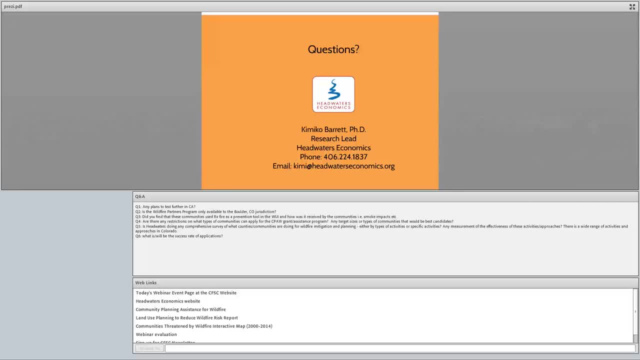 question to type in. I do want to thank the few participants who added some details, who I think are from those areas, who were able to elaborate a little bit Really cool dynamic group we had today And I will say thank you so much, Kimmy. 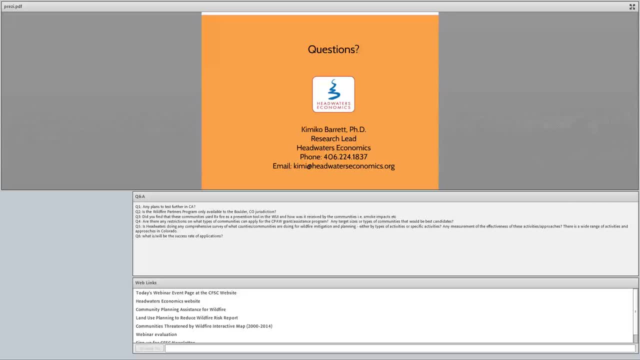 I actually didn't even know about this program, so I was so excited to hear about it, And hopefully I'll be able to share this with a number of people. I was curious too, though Is there? I'm sure this is a little bit limited on how many people are involved. 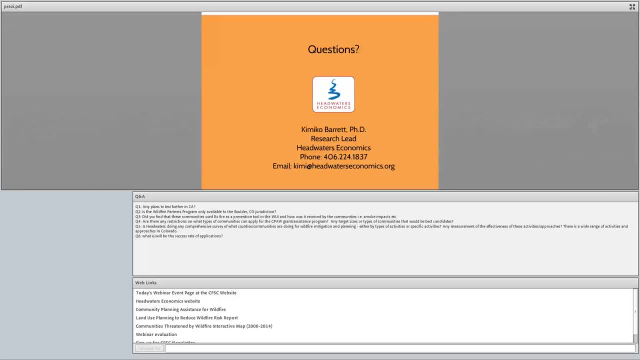 I'm not sure. I don't know how much you guys can do, So any idea of how many projects you have going forward or how likely you are to receive a partnership if you do apply as a community. So we are going to be accepting five new communities in this next phase here, 2016 through 2017.. 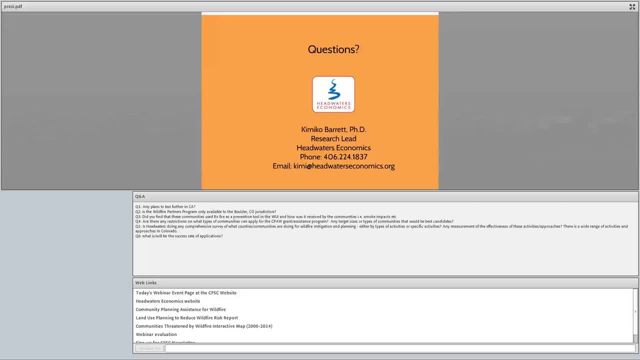 Right now we're casting a fairly wide net, but we will be limiting it to five different communities and no more, given current capacity And also we just want to ensure the success and, again, the application and implementation of our recommendations. 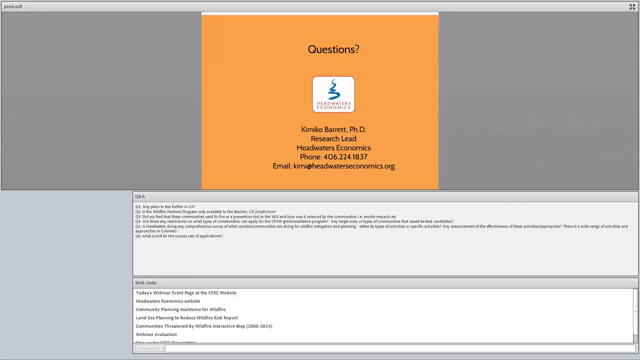 So it's very promising. It's a cooperative agreement already in place between a private foundation and the US Forest Service, who is very interested in trying to work on actual planning strategies within the WUI, And so that's Again. we really don't have a lot of limitations on the community. 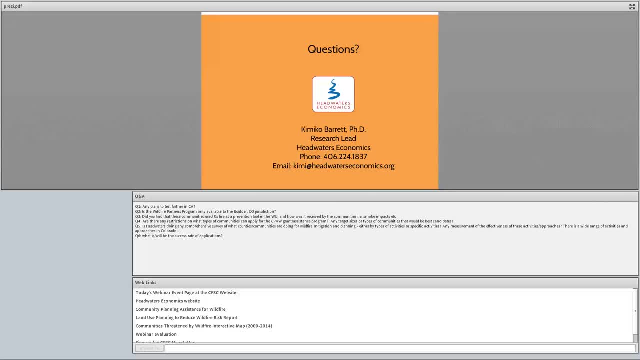 We're just trying to make sure that we're able to do that. But we do have some limitations on the community application process because we encourage it. We want folks to be part of this program And so as long as there's a couple key community contacts within each of those areas, as long. 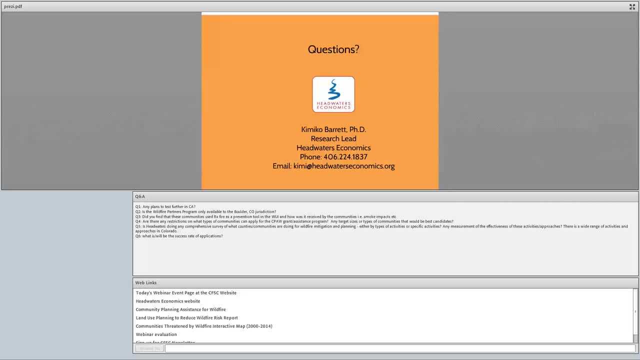 as they meet some of those criteria, then we're certainly willing to consider them as a potential applicant. And then, if we get flooded with applications, it does come down to location and who are the most promising people. So we're hoping, given the success of this past year and next year, that it will become 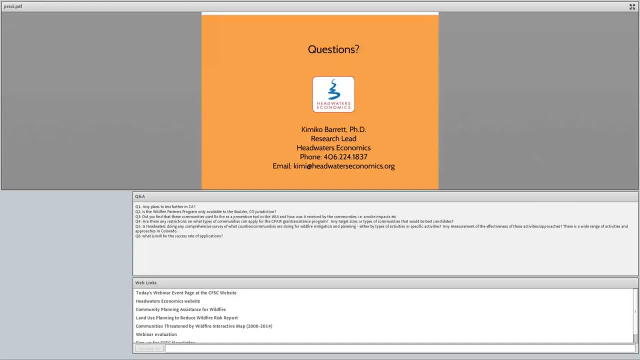 an ongoing program and then turn into its own stand-alone body in which communities in the future can apply to All right. Great Again, super exciting. So if you did register with us, you'll receive a follow-up email from me in the next couple. 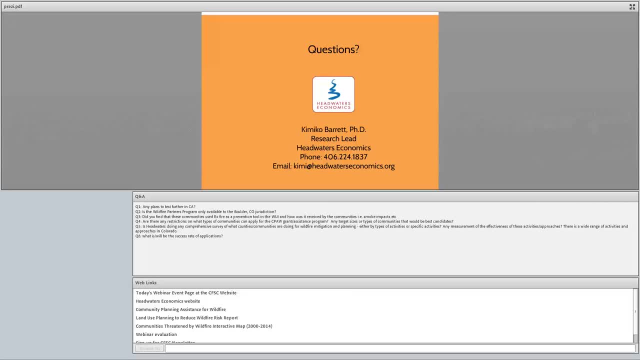 days, or at least within the next week, And that will also include the links that we talked about today, the contact information for our presenter And the recording when it's ready. So look for that And also, I should say, a link to the webinar evaluation, in case if you didn't fill it out.